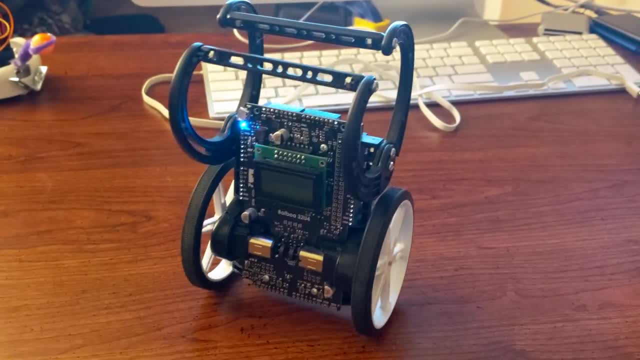 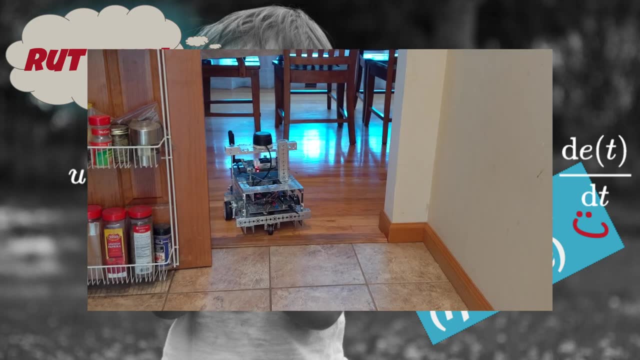 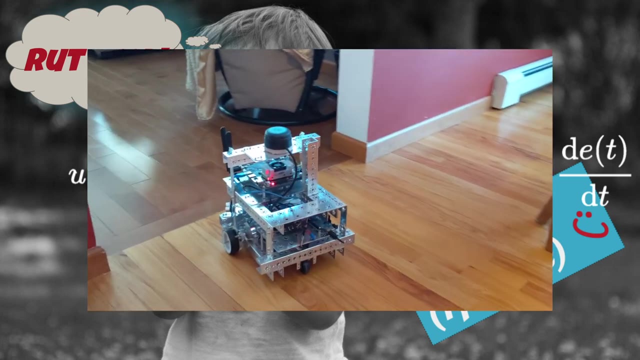 upright. You have heard me say many times throughout these videos that the math and the algorithms that we are going to learn can be applied across many different robots to solve many different problems. This same very math will both make a robot stand up and follow a wall. 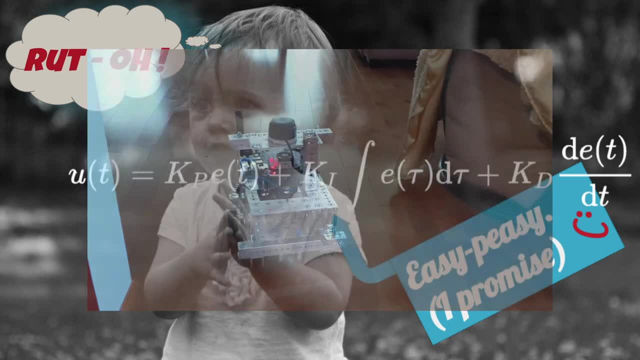 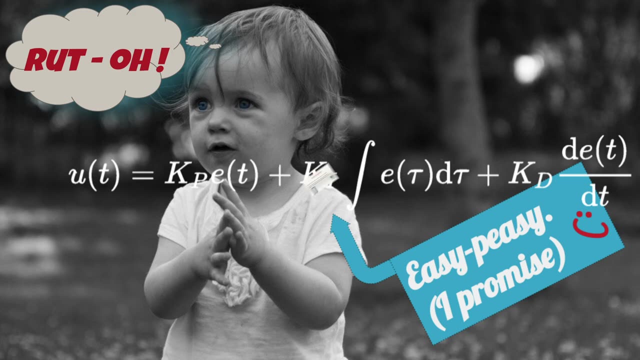 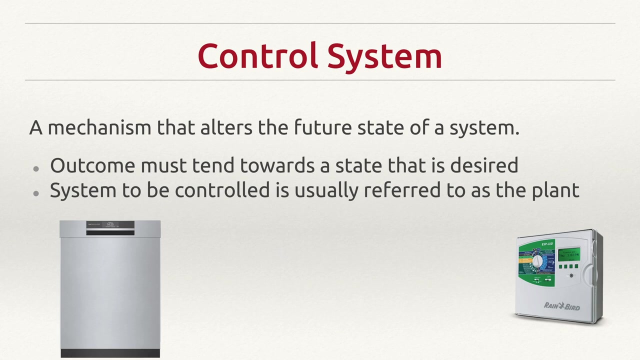 and do many other awesome things, as you will see. I want to stress that this algorithm is not that scary. We are going to break this down and make it make sense. I want to start by understanding what a control system is. A control system is simply any system. 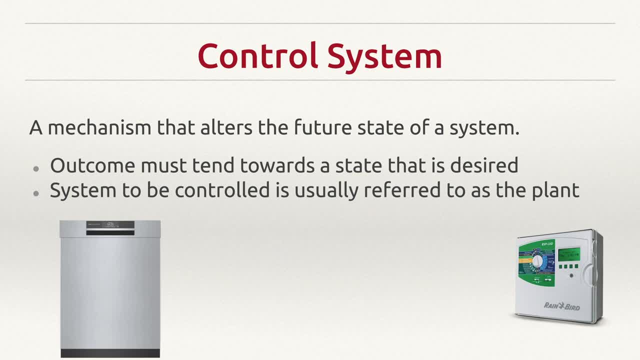 not just a robotics one that alters the future state of the system. It uses some information to do it. Now you have control systems all throughout your life. If you have a sprinkler system at your home, a dishwasher, a washing machine, a thermostat, all of these things are control. 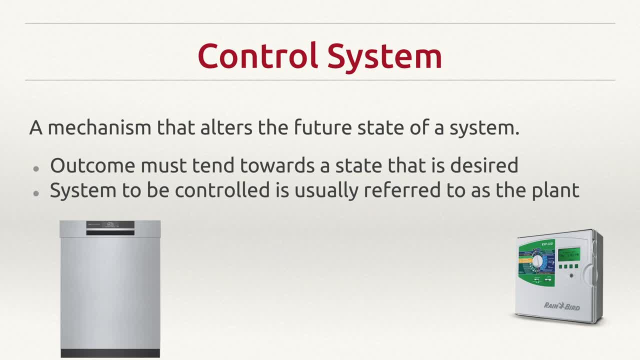 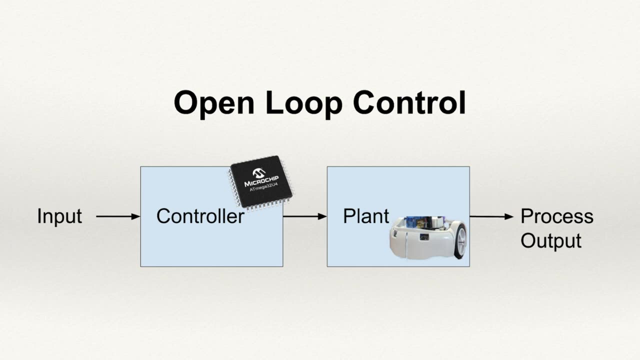 systems. In discussing control systems, we usually refer to the thing being controlled as the plant. In our thermostat example, you could think of your air conditioning unit or your heating unit as the plant. There are a couple ways that we can implement control. There is something called. 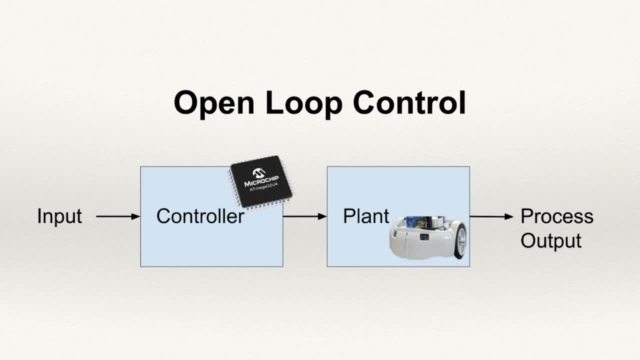 open loop control where, basically, we take some input, usually the set endpoint that we want to reach. We give it to our controller. Usually this would be our code, especially if we are working with our robots. We give it to our controller. Usually this would be our code, especially if we are working with our robots. 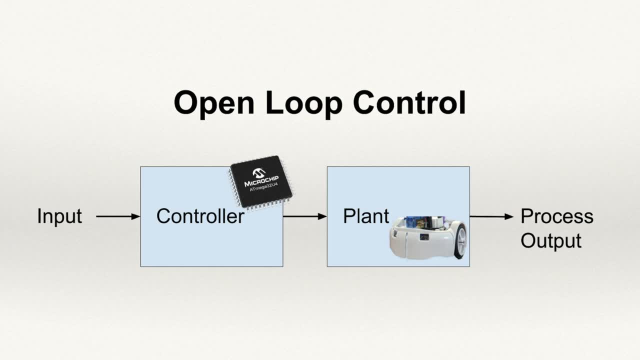 This would be our code, especially if we are working with our robots, And the controller then affects the plant, making it do the action it needs to to achieve the goal. Once we have achieved the goal, open loops control can stop. We can see this in previous things we have done. 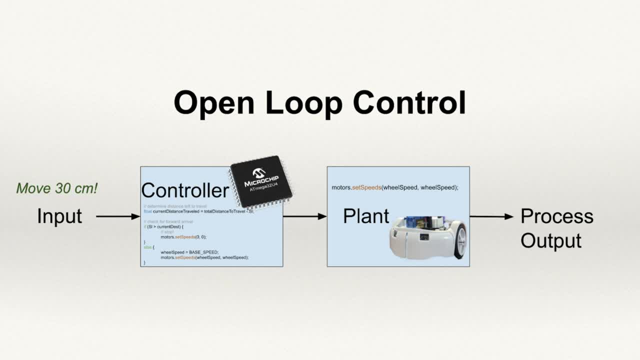 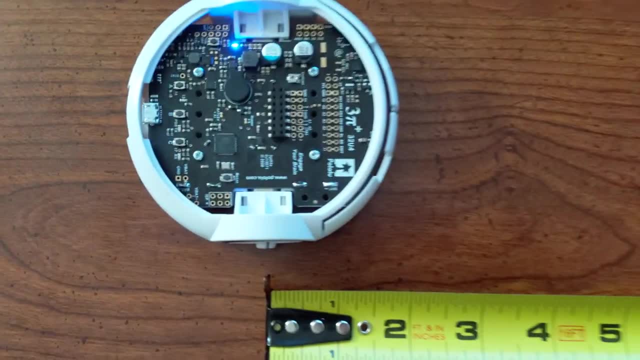 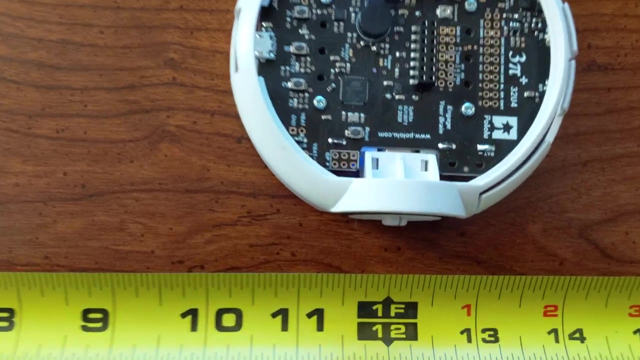 by looking at our very first algorithm, where we had our robot slow to a stop. In the most basic form of that, we were just checking our current distance traveled and comparing it against a total distance that we wanted to travel travel. Once we achieve that total distance, we simply stop the motors. This is a great example. 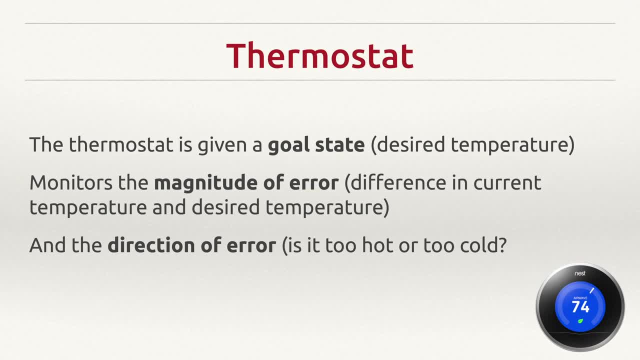 of open loop control. Now, a system that uses a different and more complicated control mechanism, although still very basic in nature, is a thermostat. A thermostat is given a goal state, just like our open loop control example. however, it monitors the magnitude of the error, which is 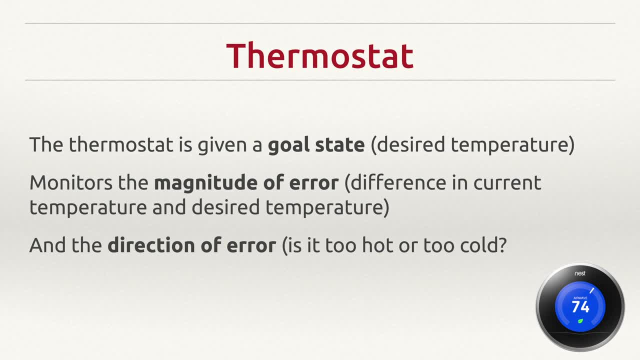 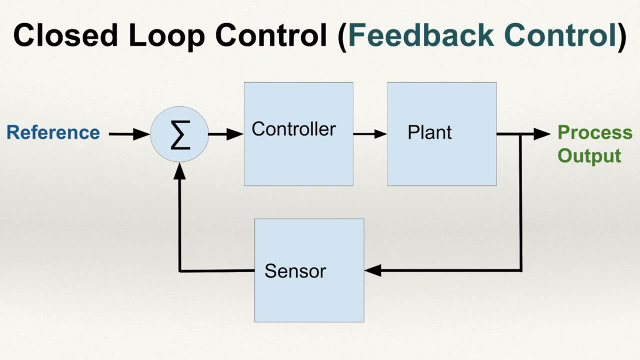 the difference in the current temperature and the desired temperature, and it also takes into consideration the direction of the error. In other words, are we too hot or too cold? Should I turn on the air conditioner or the heat? This is an example of what's known as closed loop control. 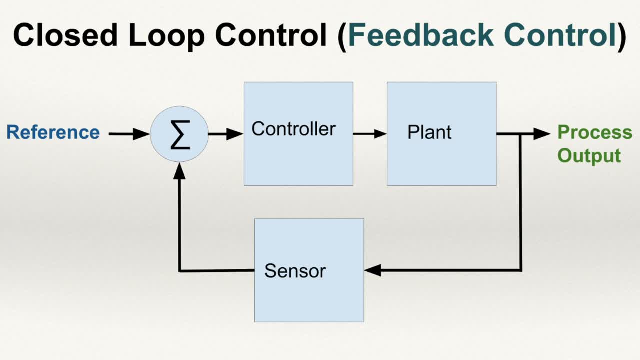 and the difference here is the fact that the thermostat monitors the current temperature and uses it as the set point to evaluate the actual temperature against the current temperature. This is an example of what's known as closed loop control. So what we're doing here is a constant comparison. In our first example, where we created an open loop, 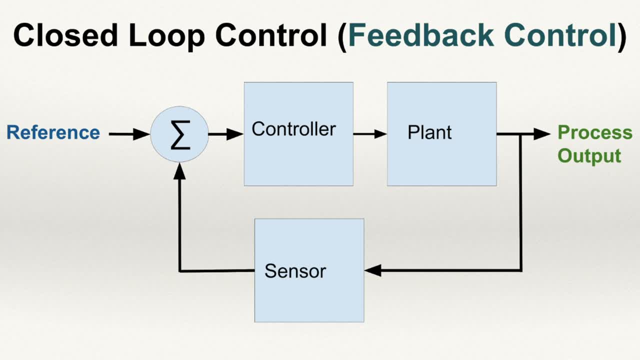 control system to slow our vehicle to a stop. our goal was to reach a certain distance, but we did not take into account any other variables. We did not take into account if I picked up the robot and moved it, or if I bumped it, or if there was a wall in the way. None of 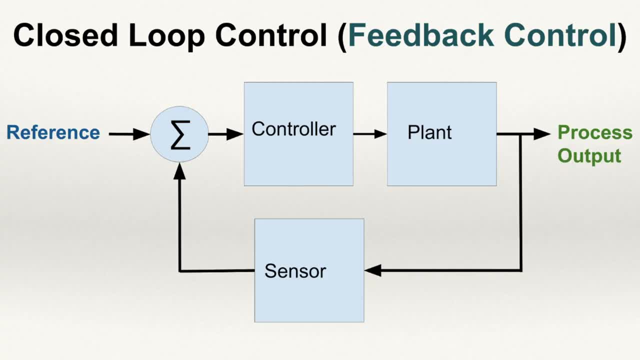 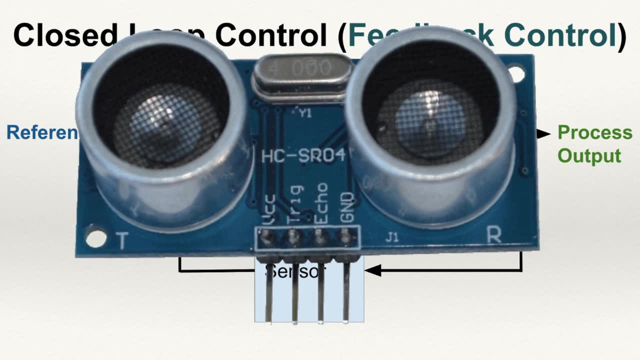 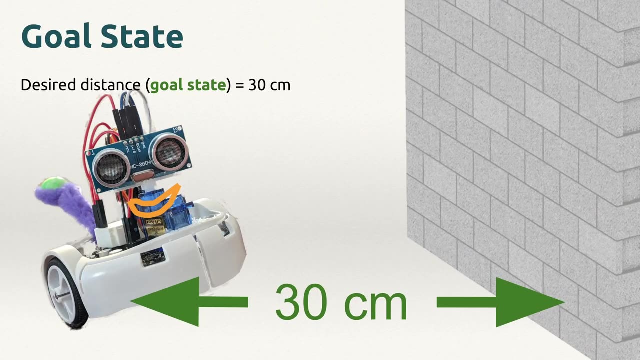 that mattered. All the robot knew was how to move 30 centimeters forward In closed loop control. we take in some information from the environment using our sensors and then use that to evaluate, just like a thermostat does. Let's now see how we can apply this to our robot. if we wanted to say: 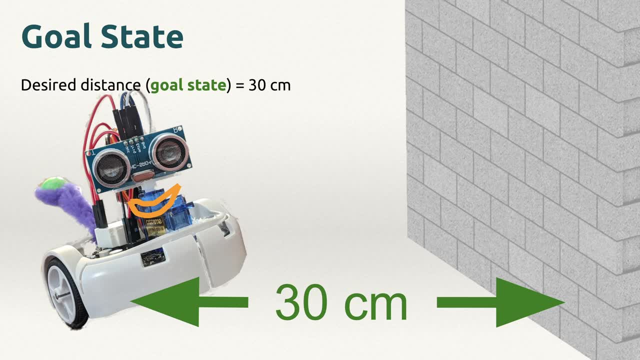 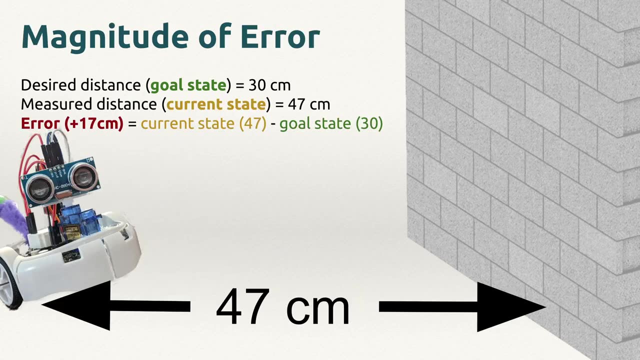 follow a wall. Let's say that our desired distance, that we want the robot to always stay from the wall, is 30 centimeters. Then let's say that we use our ultrasonic sensor to measure the current distance that the robot is from the wall. Now, in this example, let's pretend that the robot 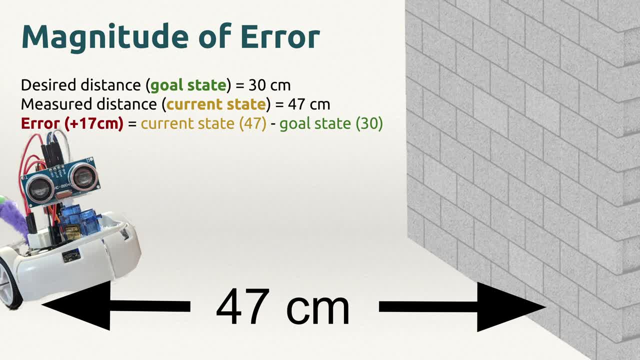 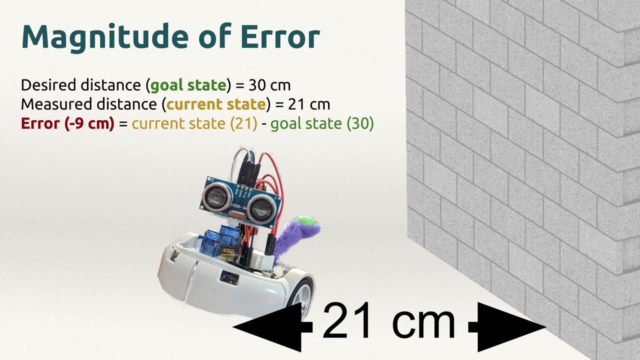 has wandered a little bit further away than we would like and is 47 centimeters away. That means that our error is 17 centimeters. It is the difference of the current state and the goal state. Now we could also be too close to the wall In that example. our current state is 21 and our 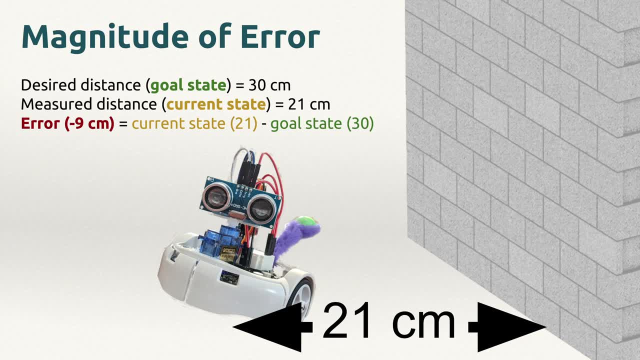 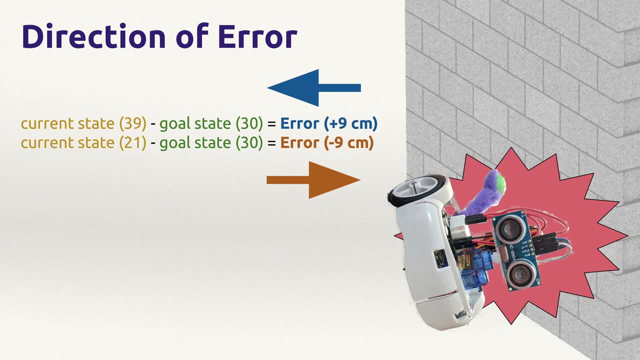 goal state is 30, so our error is actually a negative number. It is negative nine, Knowing whether the error is positive or negative, in our case for the wall following robot, is our direction of error. Just like the thermostat can tell you the temperature is too high or too. 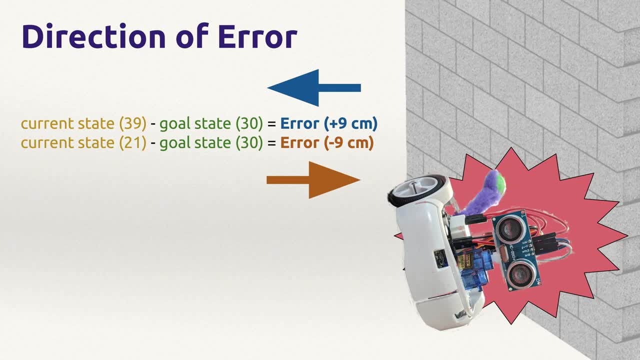 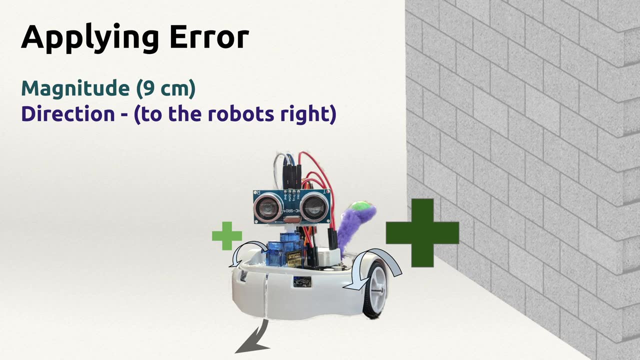 low. this now is going to tell us whether the robot should go left or right to compensate. So let's see now how we can apply both the magnitude and the direction of error to achieve the goal of following the wall. Let's say that our robot here has a base motor speed of 50,. 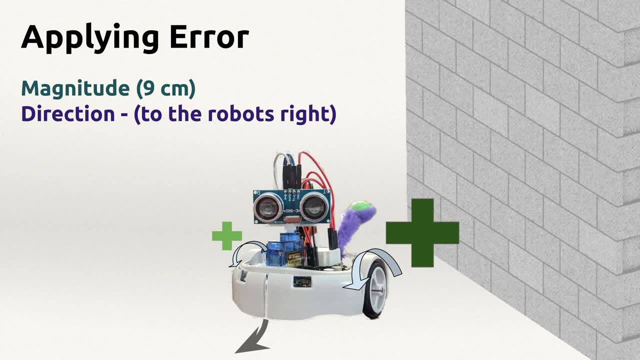 so if there's no error introduced into the system and the robot is 30 centimeters from the wall, he will drive in a straight line at a base speed of 50.. Now let's say, at the current moment the robot does have an error of 9 centimeters, so the robot is too close to the wall. What we can do now: 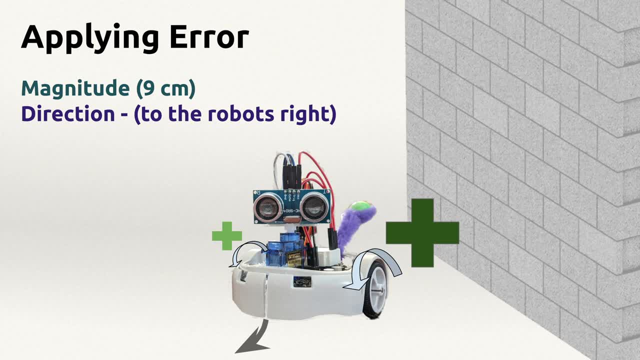 is, apply that magnitude of the error to the plant or our wheels by, say, giving a positive magnitude to one wheel and a negative to the other. So if we had a base speed of 50 and let's just say that we just take the error, we could apply positive 9 to the robot's left wheel here on the 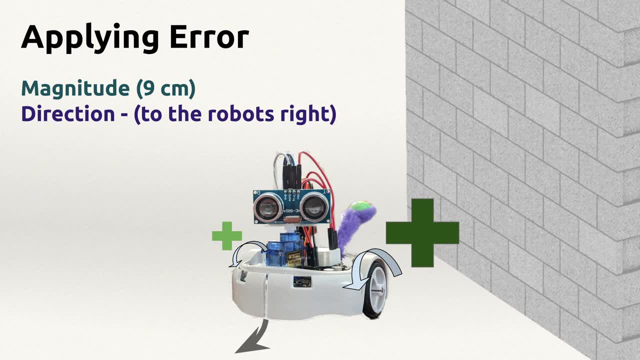 right side of this image and negative 9 to the robot's right wheel, and the robot would naturally turn to its right. this would have the robot moving away from the wall. The motor speeds on the right wheel there would be 41 and on the left wheel, closer to the wall, would be 59. So you can. 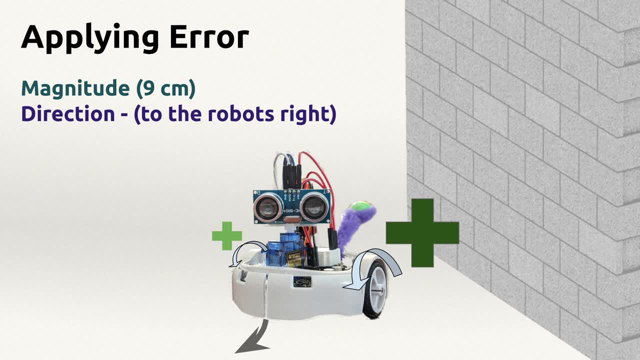 that the faster speed would push the robot off to the right. Conversely, what if the robot's error was positive? What if the robot was too far away from the wall? Well, in that case we could just simply reverse it. We would apply the 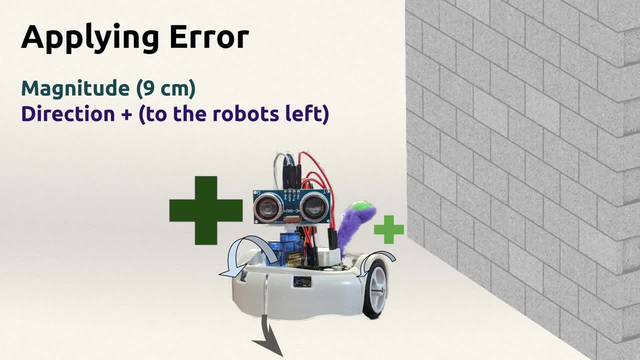 positive number to the right wheel and the negative number to the left wheel, So we would end up with a 59 on the right wheel and a 41 on the left wheel, causing the robot to turn left. The great thing about an approach like this is that the 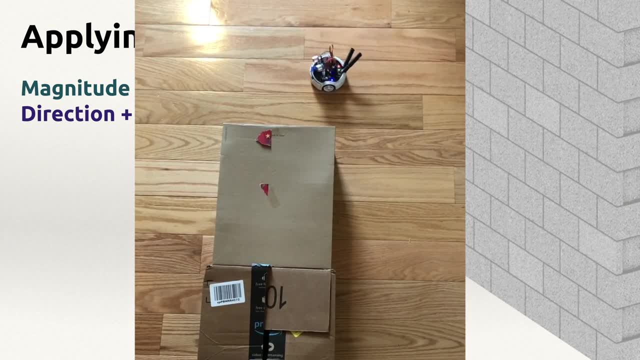 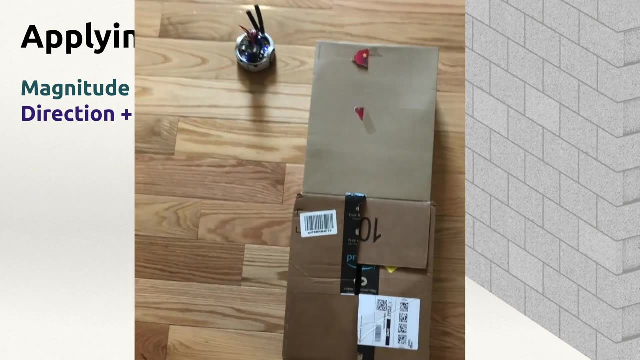 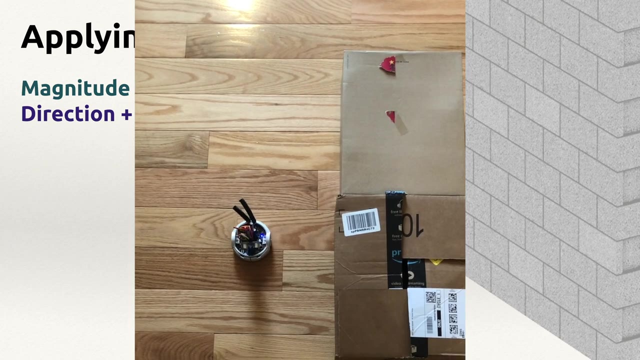 magnitude of the error is going to dictate how quickly the robot turns. So if the robot is far away from the wall or very close, it can react more quickly, and as it approaches the goal it's naturally going to act more slowly. If we only have an error of one centimeter, then the power to the wheel that it 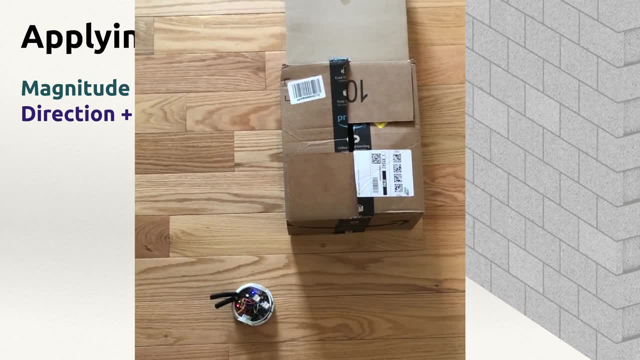 needs to compensate is only going to be plus one, and the other wheel is going to be minus one. So we're in a 49 and 51. This is a little bit of a disaster, but it's not a big deal. It's not a big deal, but it's not a big deal. 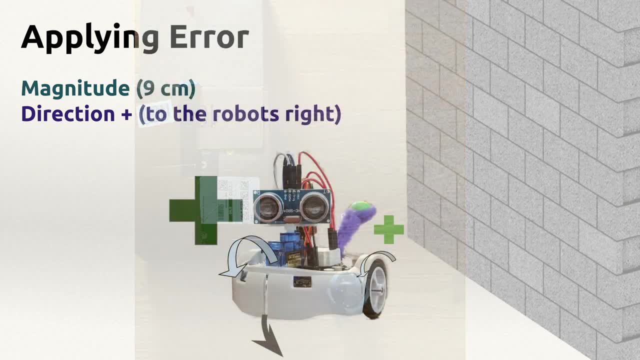 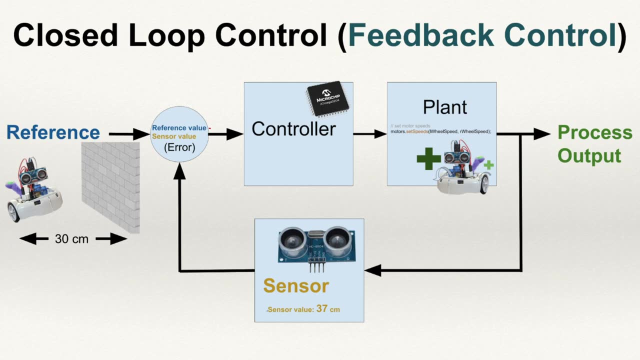 difference in wheel speed, but not enough to make the robot look jittery. So now let's see how we can apply closed-loop control to our robot to achieve this goal. We know that our reference value, and the value that we're going to use as monitored by our sensors, is going to be the distance, So we know. 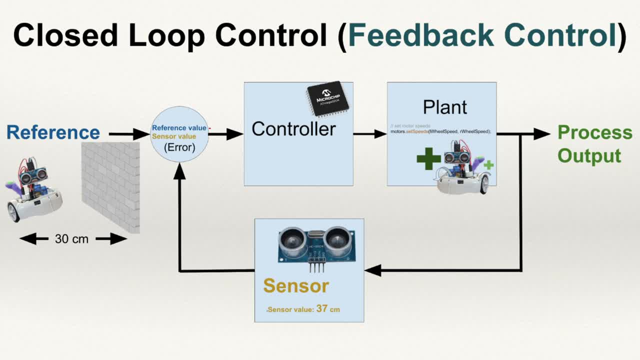 how to do that with our ultrasonic sensors. If you haven't yet seen it, please check it out in the videos here- And we're going to use that error to run into our controller. Now the best way to do that is to go to the controller and 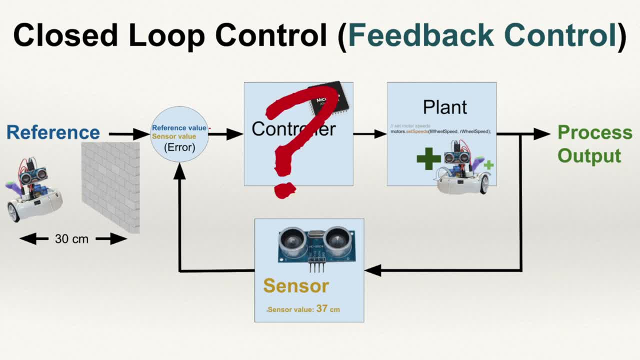 the big question is: what algorithm should we use to apply to this error to affect the output that we want on the plant? So we can see here on the plant that we want to have the output affect the set speeds method of our motors. But what do we do there? right, 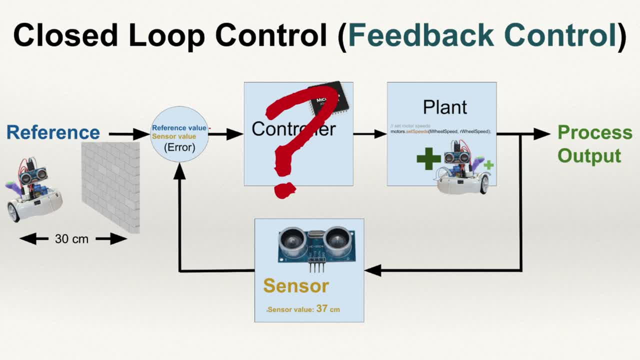 What is this magic algorithm that we're going to use that's going to make the robot glide across and follow the wall, just perfectly Well, the answer is that PID algorithm that we talked about earlier And, as I mentioned, you can use this algorithm to solve many problems, not just. 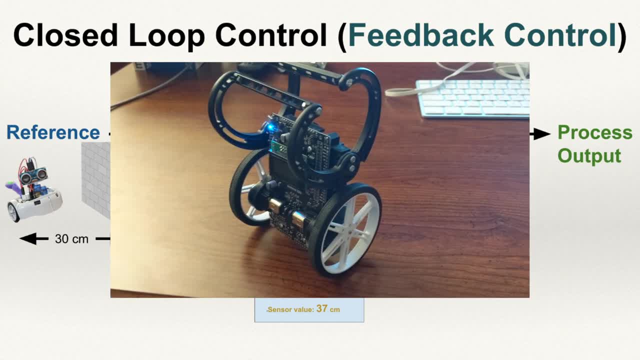 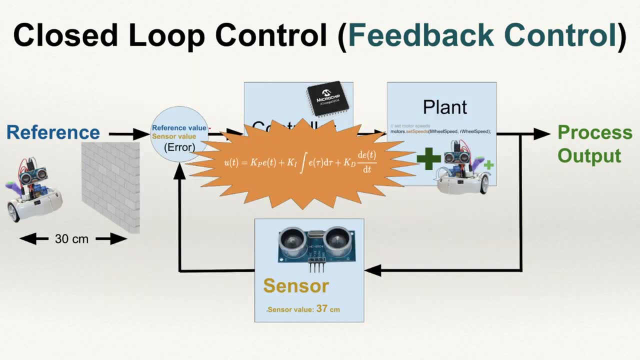 wall following. In fact, I'm going to use an example which is a little bit harder throughout this video, where I make a robot stand up. The key to understanding how to use a PID is to understand that you simply apply the math. the same way. 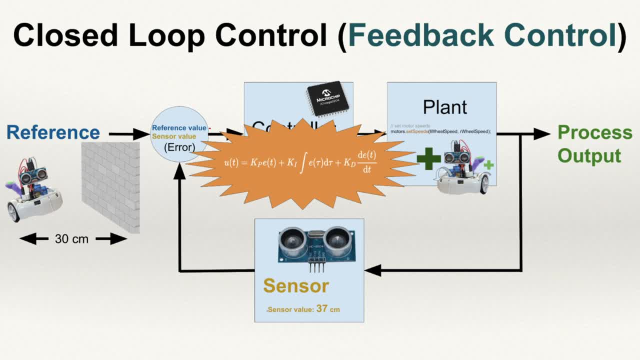 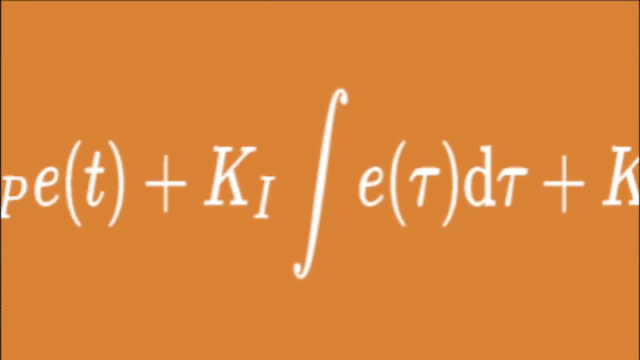 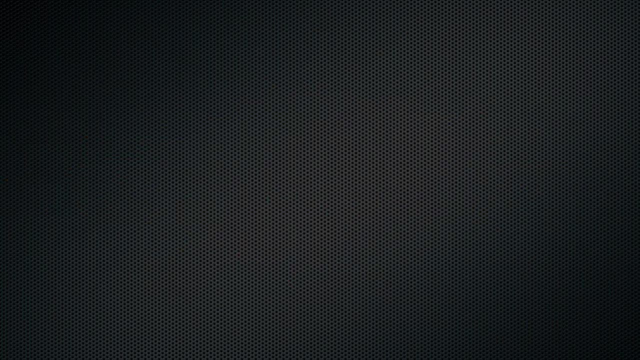 to solve every problem. but then there are three tuning constants that you use to affect how the robot reacts to the PID algorithm. So here it is in all of the PID algorithms. I promise it is not as scary as it looks. I know that it can be intimidating and it 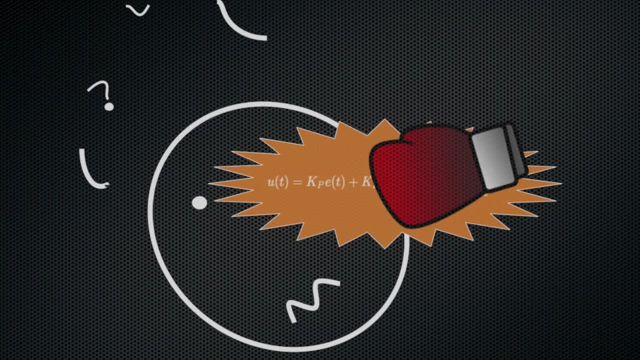 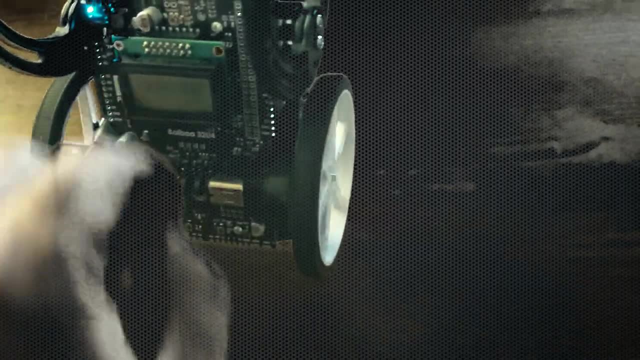 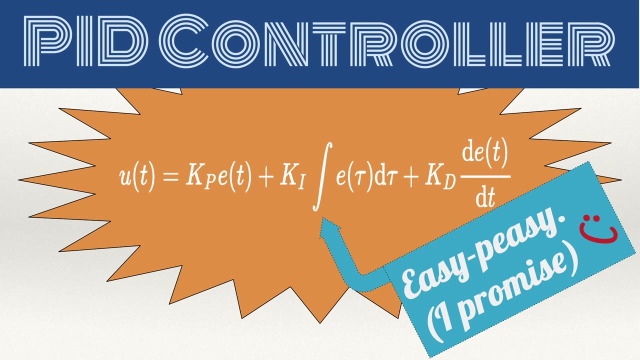 might even feel like a punch in the face when you see these mathematical algorithms, but breaking this down, it's actually just three simple equations that make robots do magic things, So let's get started. Okay, let's break apart this PID algorithm now and see how it works. As I mentioned earlier, 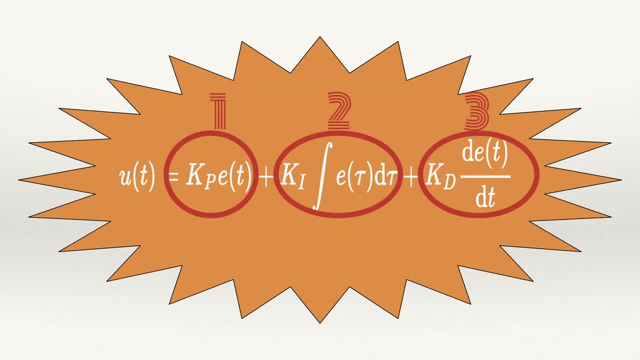 it is not as bad as it looks. In fact, understanding first of all that it is just three simple equations that are summed together is the first step in understanding it and making it simple. Let's look at each of the three, one at a time. The first is proportional. 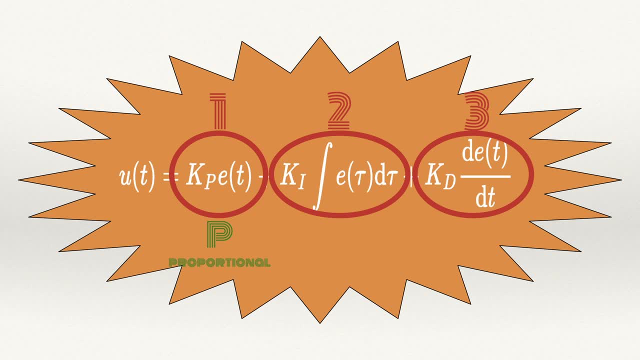 This is actually a simple multiplier of the error. We're going to talk more about the details in a moment, but it is quite simple. It is also the most commonly used portion of the PID controller and it is the one that I will usually recommend that we start with. 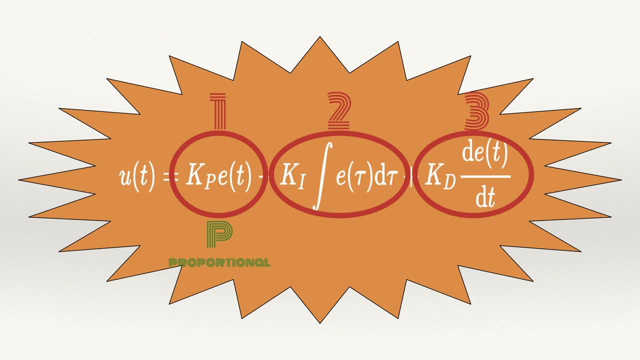 because it has a very linear output and it's easy to understand. So let's get started. The second one is integral. This is the summation of error, and this has a really good effect when you want to get the robot to get rid of what's known as steady state error, As 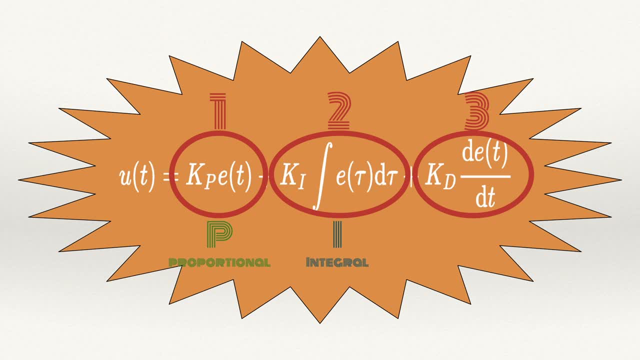 the robot is close to the goal, there's not going to be a huge proportional response and there might not be enough proportional response to push the robot back to the goal. Or if you increase the proportional response, the robot might overshoot. However, those 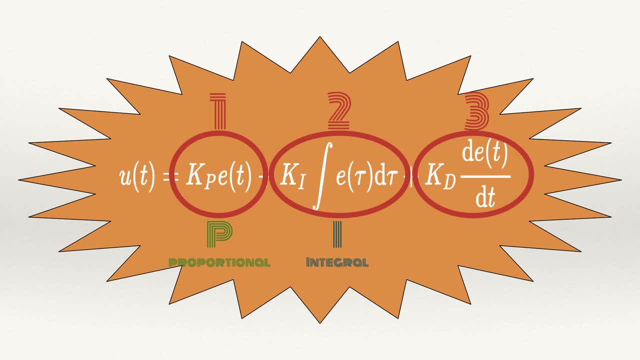 little amounts of error, When you sum them up And then multiply them, will have a greater effect, and this is what integral does well. The third one is the derivative. This is actually the change in error. Now, this one is very interesting because it actually counters the other two. If you have a robot that's standing 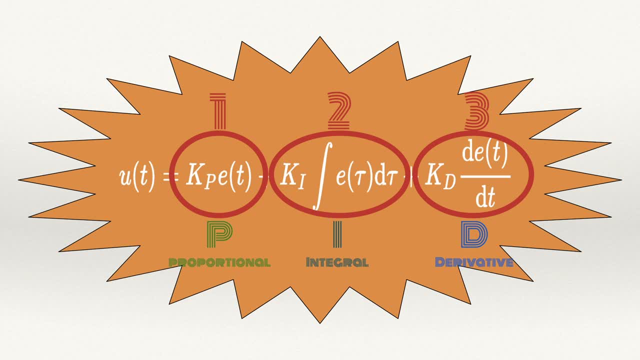 up and it's relatively straight and steady, then you're going to have a very low proportional and a very low integral, because the robot's been standing successfully. However, if I push the robot In an effort to knock it over, the change in error is going to get very high, very fast. 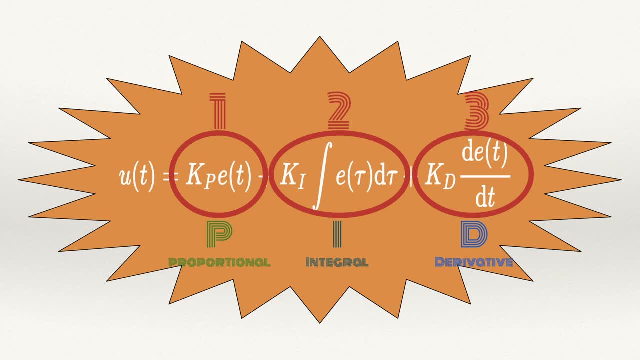 It's going to take time for the integral to wind up and the proportional is going to be responding the more the robot rolls over. The derivative now is going to actually act to cushion the response on the proportional and integral. It's actually a counter. so 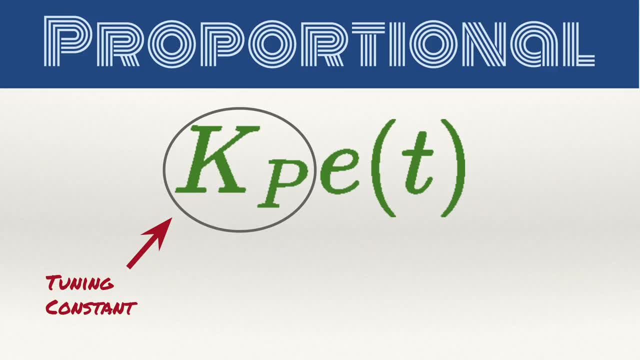 to speak to what's going to be a large response. Let's look at each of these now and see just how simple they are. I mentioned earlier that there are three tuning constants in. there's one for each, So the tuning constant for proportional is known as kp. This is just a number that we 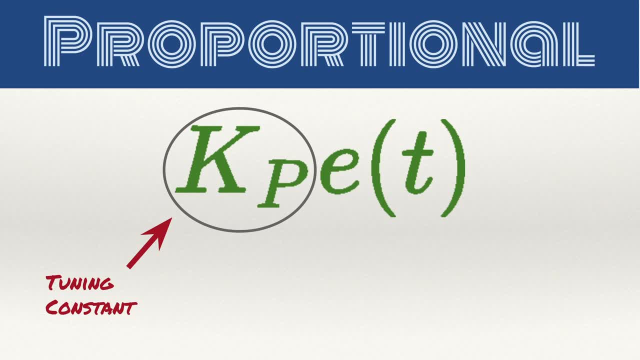 pick. The larger number we pick, the more the proportional output will be. The smaller number we pick, the last the proportional output will be as part of the overall PID. So let's just pretend that we pick a tuning constant of 10.. Now the E just stands for. 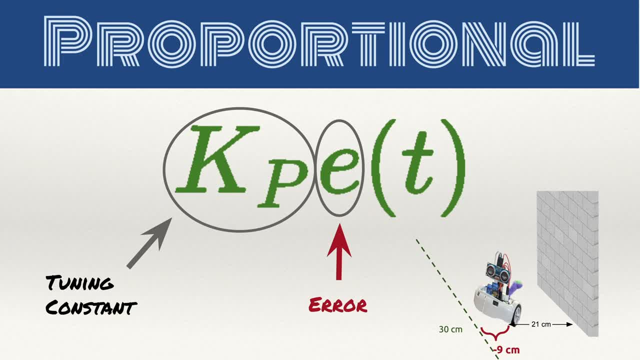 our error. So if we imagine that at any given moment in time, say, our robot has an error of negative nine, we could multiply that by our tuning constant. so KP times error here would just be negative 90. that's it, in fact. the last part of this is time now. 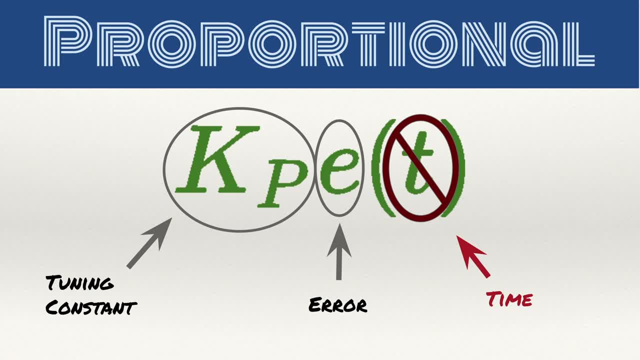 this is optional and that's important to keep in mind. if your controller has a very steady Hertz of how often it refreshes- say that every 10 milliseconds your PID controller runs- then you don't need to necessarily multiply by time. all you're going to do is make the amount of the output 10. 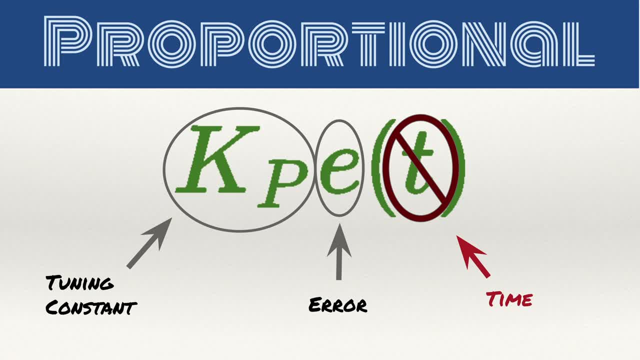 times larger. when this is useful is if your PID controller, say, does not have a very steady rhythm. let's say that between time 1 and time 2, 10 milliseconds elapsed, but between time 2 and time 3, 20 milliseconds elapsed. you would want that second gap in time to have twice the 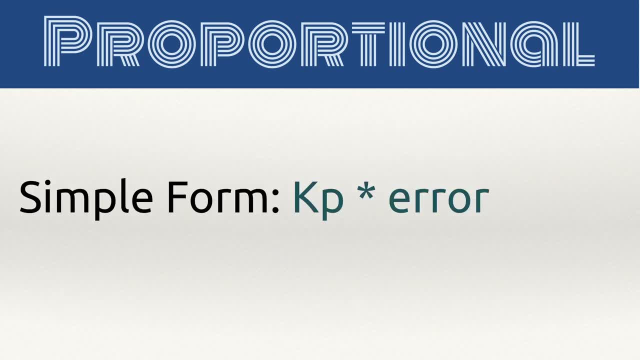 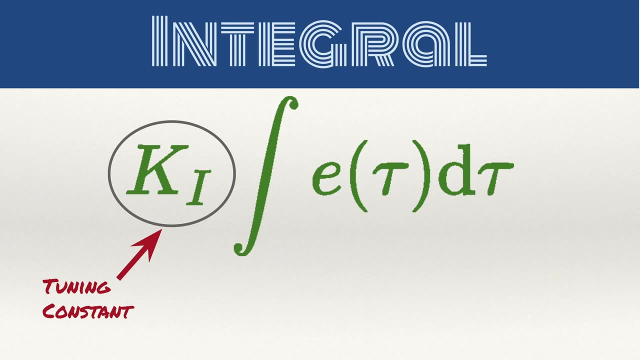 effect, and that's when multiplying time is important. this is the simple form. this is it. it is just your tuning constant times. the error. now let's look at integral. now, this one is just slightly more complicated, but it's not honestly complicated at all. again, we have our tuning constant, which is KI. this is the. 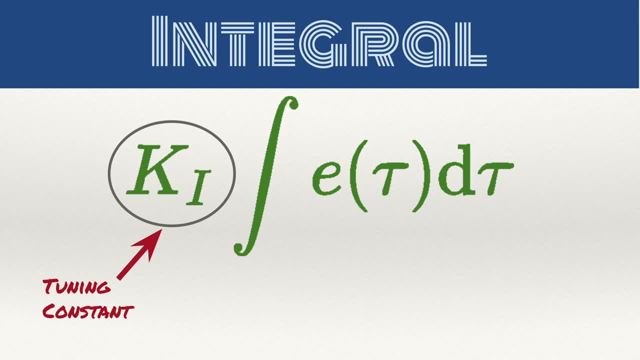 multiplier that we're going to use for the integral portion, again affecting the output of the integral. a higher tuning constant will produce a higher output. this symbol is just the integral sign and we are just denoting that we are going to take the integral of summation of. 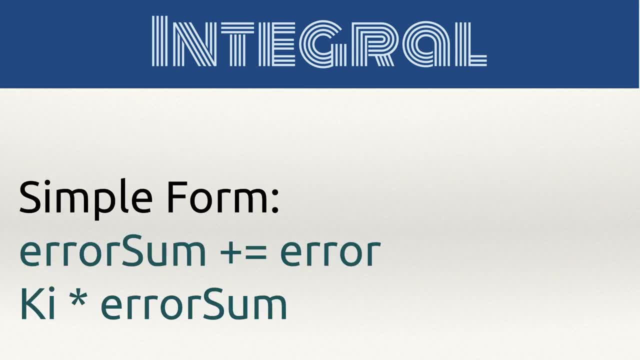 the error here. Let's look now at the code to see how this would look. So again, this is not much harder. We simply have a summation of error that we're adding the current error to to keep track of it as it grows, and then we are just simply multiplying it by our constant, If we imagine. 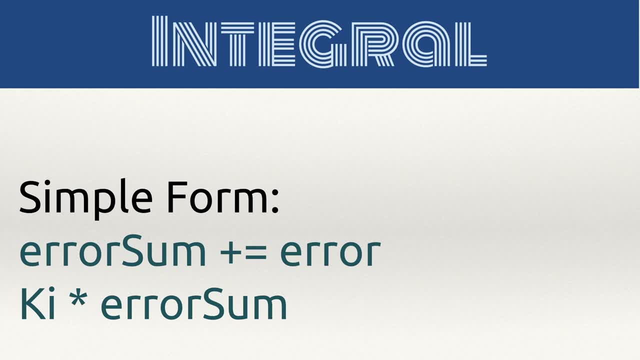 that at time one we had an error of 10, and this is the first time measured. then our error sum would be 10, and the output, if our ki was 10, would be 100.. Now let's say at time two the error is 5.. 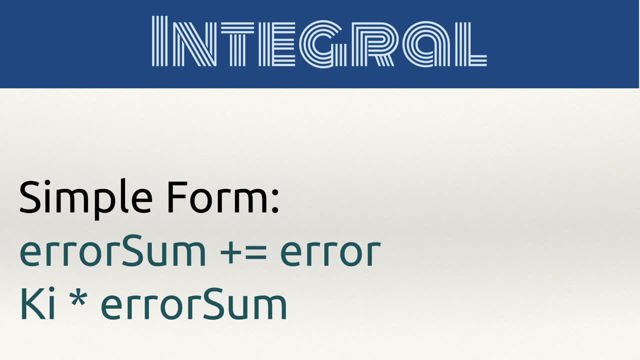 Well, we would add that to the 10,, making our error sum 15, and then our ki of 10 times 15 would give us an output of 150.. Let's imagine that at time three our error is actually negative 15.. 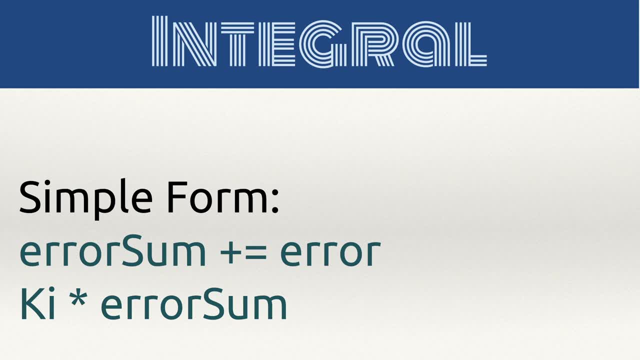 Let's say that our robot went past the goal and in the other direction. Well, that's actually going to reduce our error sum back down to 10 from 15, and now, when we multiply it by ki, we're going to get a total output for integral of 100.. One important thing to know about integral is that 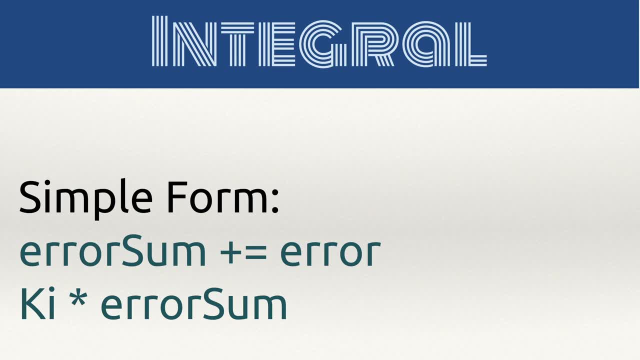 it can cause what is known as windup. You can end up with a large number in your summation that will have a large effect on the robot. A very common situation is when you have a robot that has a large number in your summation and you have a. 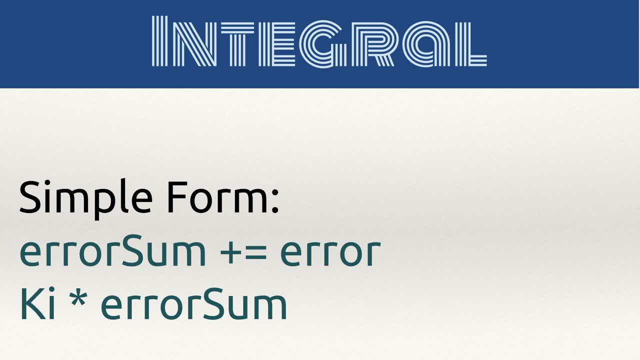 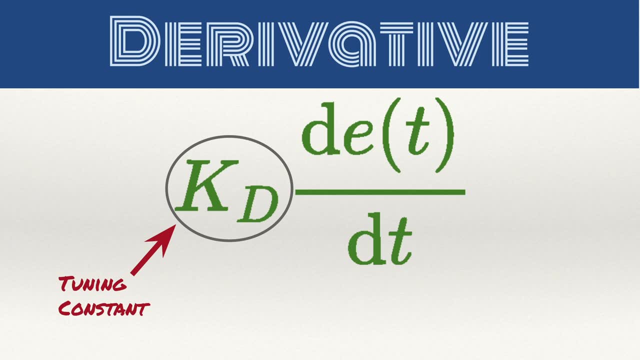 large number in your summation and you have a large number in your sum, So what we can do is simply to provide limits to how much summation can happen. Derivative is just like the other two. There is a tuning constant known as kd. What it is multiplied by is now the difference of the 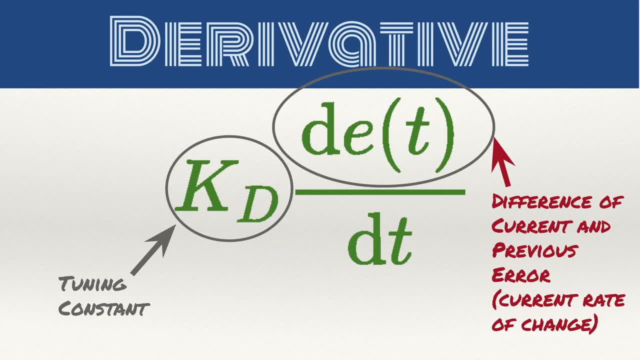 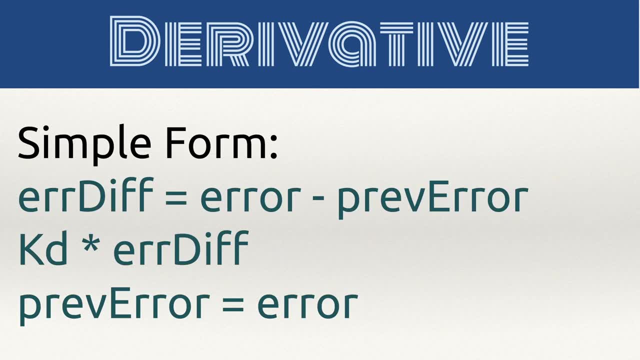 current and the previous error. Now you can also divide this by time, but again, if you're leaving time out, then you don't have to do that. So here we go with the simple form of this equation. We have the difference of the error, which is just simply. 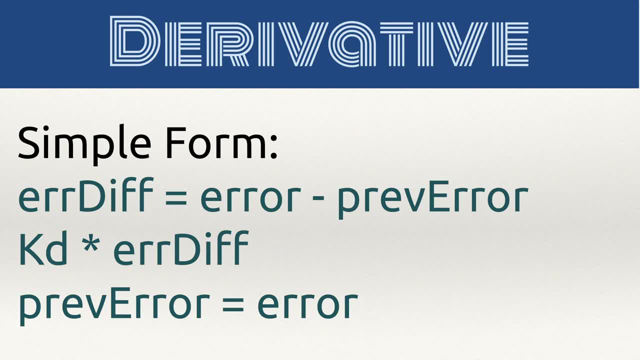 our current error, subtracting the previous error, and then we multiply it by our constant. Lastly, we're remembering to update our previous error with this error, so on the next go around, we keep track of it And that's it. This is all three of them When you add the result of these. 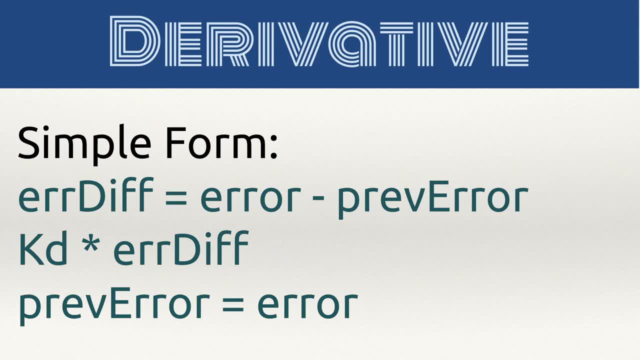 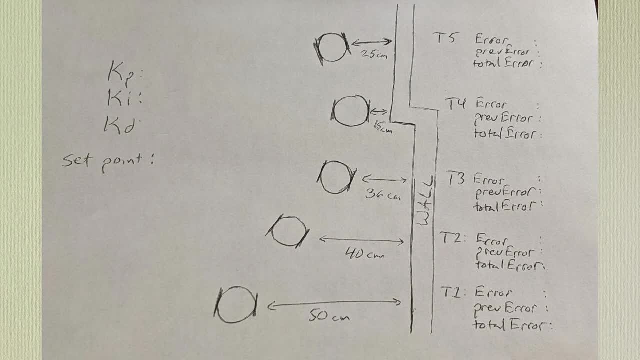 three together you get the total output of your PID. I find the most useful way to understand these algorithms is to actually visualize it by creating a handwritten verification. So what I have here is an illustration of a robot trying to follow a wall. You can see that the robot has five time periods- t1, t2, t3,, t4, t5, at which it 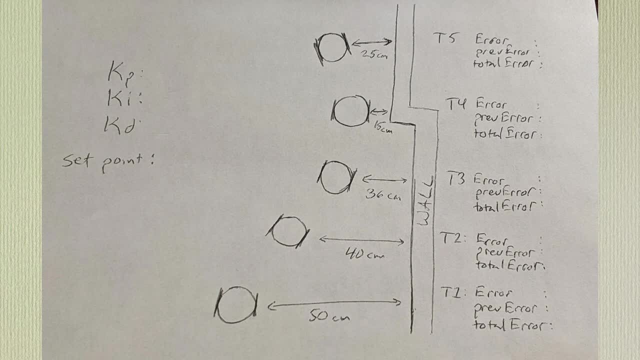 is different distances from the wall. We also on the left side have some space for some constants: kp, ki, kd and a set point. These are going to be the tuning constants and the physical constants for which we've set our plan, such as the set point, and we're also going to add in a base wheel. 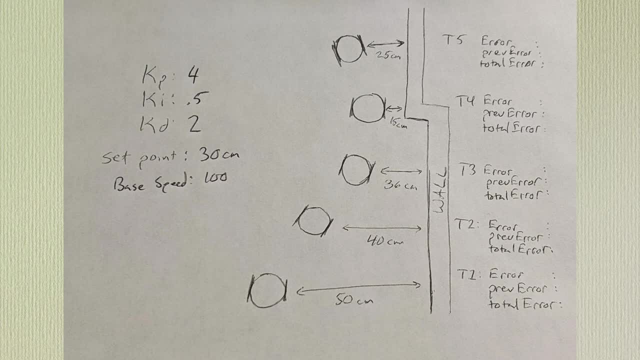 speed as well. Let's fill in some of our points here with data. So our three tuning constants, kp will be 4, ki will be 1, half or 0.5, and kd will be 2.. We also have the set point, or goal. 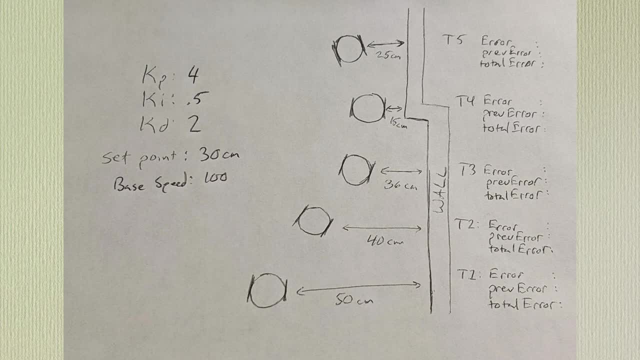 state of 30 centimeters. so we want the robot to be 30 centimeters from the wall And we're setting the motor base speed at 100.. So we have a set point or goal state of 30 centimeters, So we want the robot to be 30 centimeters from the wall and we are setting the motor base speed at 100. 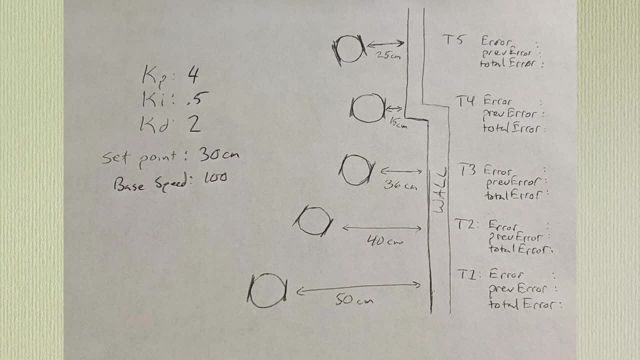 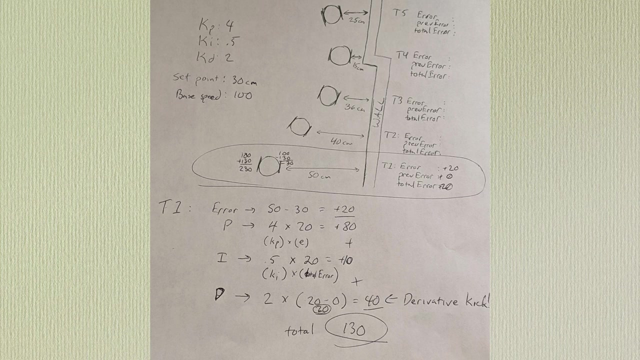 And we're setting the motor base speed at 100. So this just simply means if there was no error and the robot was moving ahead, it would move straight ahead at 100 base speed for both wheels. So at time 1 now our robot is 50 centimeters from the wall To determine our error. 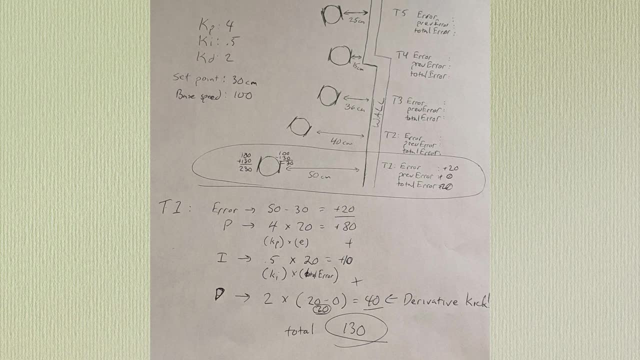 we know that we take the current distance, which is 50,, subtracted from the goal or set point, which is 30, and that means that we have a difference of positive 20.. So our error is 20, and our direction is positive. Now we're going to take this error and we're going to apply it. 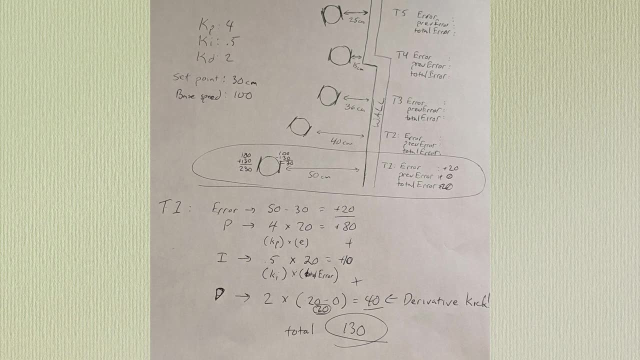 to see what we're going to do through our PID algorithm. So our proportional, our p factor, takes its constant of 4 and multiplies it by the error of 20, and that gives us back the value of 80. Now our integral is 1, half for its constant, so it's 0.5 times the error. Now remember the. 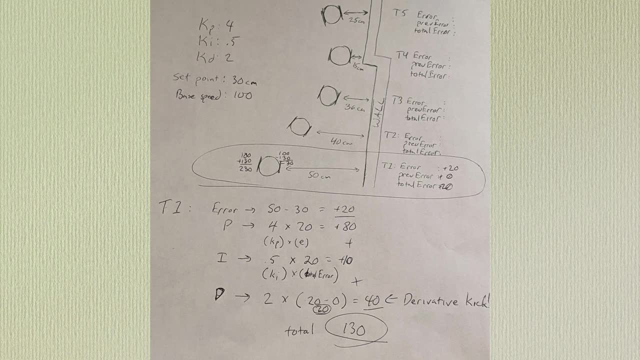 integral is using the total error, but since this is time 1, our total error is still 20.. There we have a value of 10, since 0.5 times 20 is 10.. Our derivative now takes its constant of 2 and. 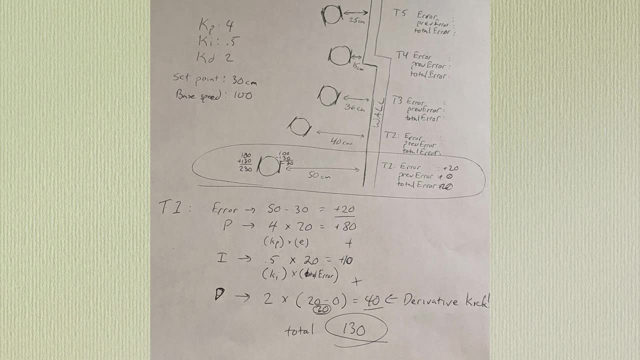 multiplies it by the difference of the error. Now this is a little bit tricky on the very first go, because there is no previous error. The previous error is 0. So what we end up with is a current error of 20 minus a previous error of 0, which leaves us with 20.. This actually causes a big 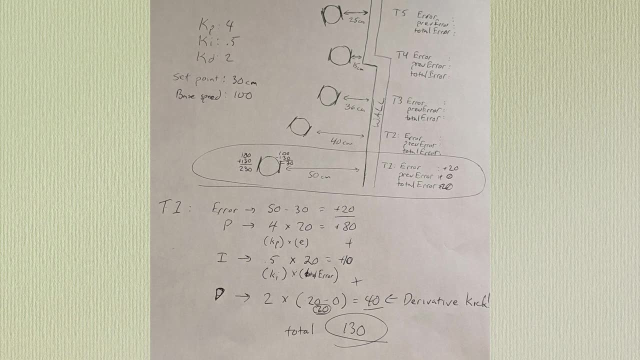 derivative function much bigger than we would normally see. So we have: 2 times 20 equals 40. This is also known as derivative kick. You might see this on the very first time that your robot reads, since it has a previous error of 0. 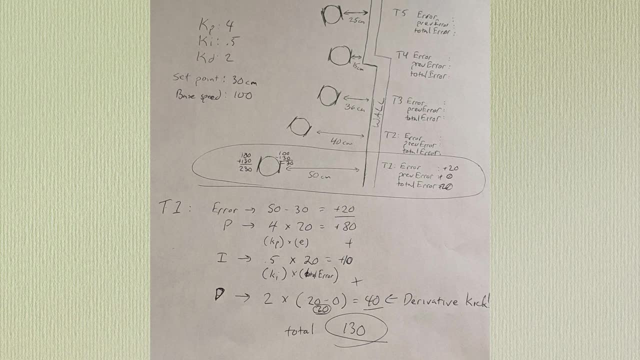 or if the set point is changed. So when we total these up, remember you take the value of the output of all three components of your PID and we add them together, we get a total of 130.. Now we're going to apply this 130 to the wheels, So we have our base speed of 100.. So the left wheel gets 100. 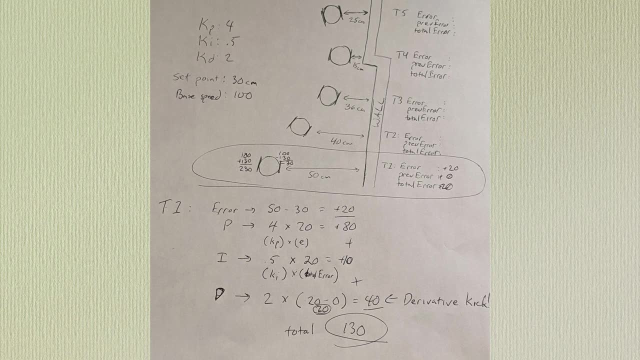 plus 130 as the force speed of 230. And the right wheel gets 100 minus 130 for a value of minus 30. So this means that the right wheel is actually rotating backwards slowly and the left wheel is moving forwards more than twice as fast. 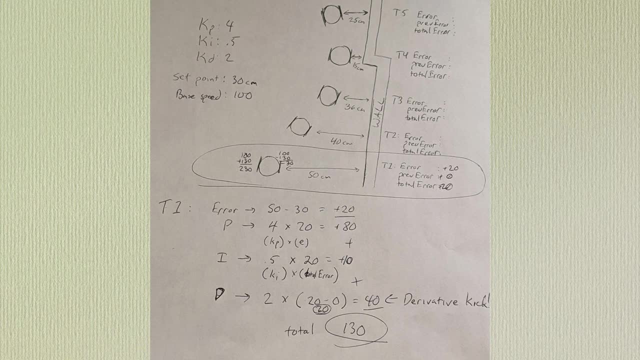 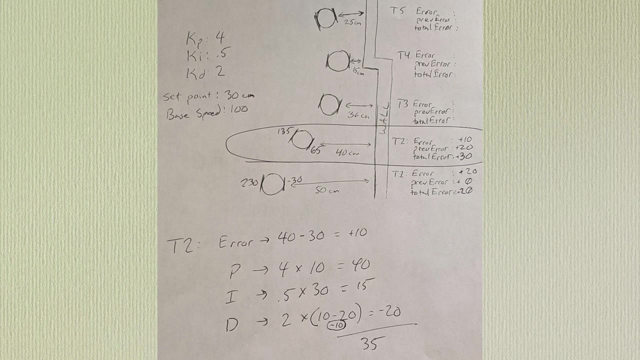 as the base speed. This means that our robot is going to turn relatively aggressively in towards the wall. Moving on to time 2, now we can see that the robot is 40 centimeters away from the wall, from the 50 centimeters it was in time 1.. Now our error is 10, since the current distance of 40 minus. 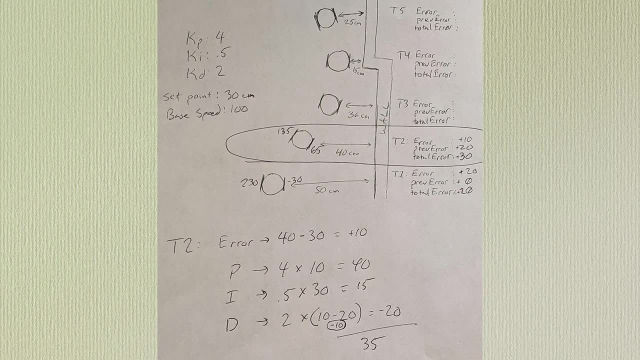 the set point of 30 equals 10.. So we're going to use our error of 10 into our PID controller. So our proportional uses its constant of 4 times the error of 10 and gets back a value of 40. The integral. 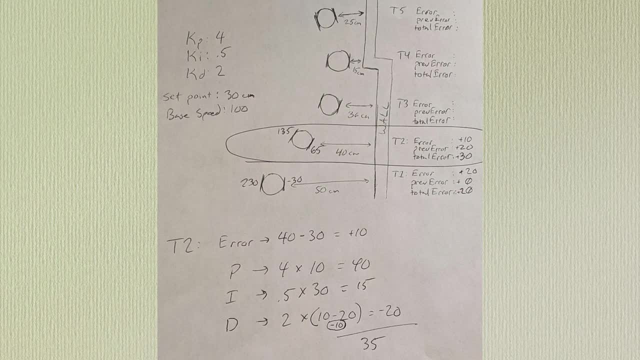 now has something to keep track of as a total besides the current error. The total error is 30 in the previous go around at time 1, plus the current 10 in time 2.. So our 30 times the point 5 gives us an interval of 15.. The derivative now is actually starting to act like a derivative. 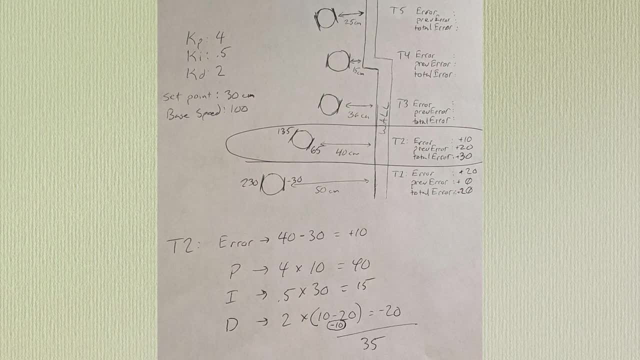 So its constant is 2, but it is multiplying it by the current error of 10 minus the previous error, the difference of 20.. So that gives us a value of minus 10.. So when we multiply our constant, that gives us a total for this of minus 20.. Now you might remember: 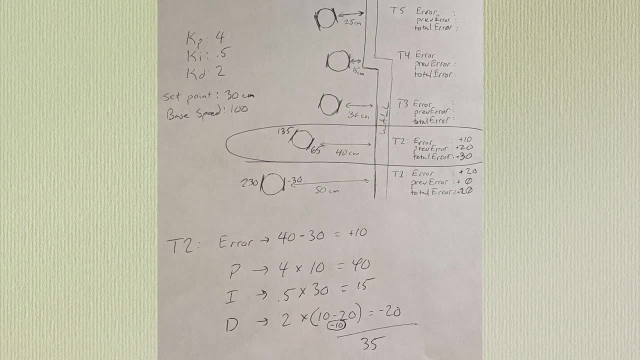 earlier I mentioned that the derivative actually acts as a buffer. It actually slows down the proportional integral by kind of being a counterweight. So we have a 40 plus 15. so 55 minus 20 brings us back down to 35. We then apply the 35 to the left wheel because we're still too. 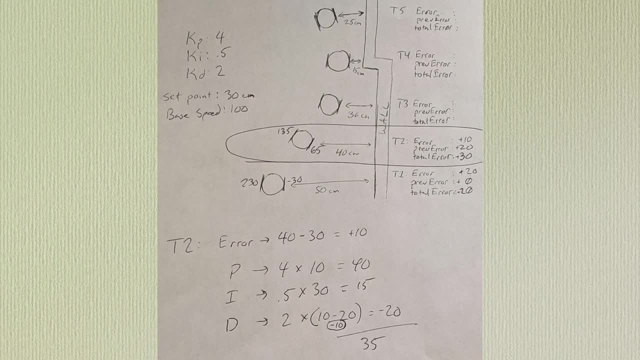 far from the wall as positive and a negative to the right wheel. so now we have a left wheel value of 135 and a right wheel of 65. You can see that although the robot is still turning towards the wall, it is doing so less aggressively. 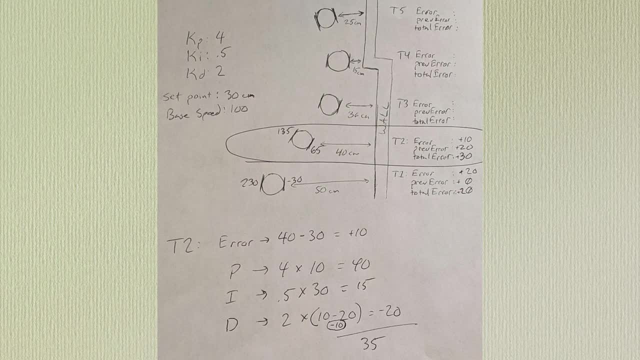 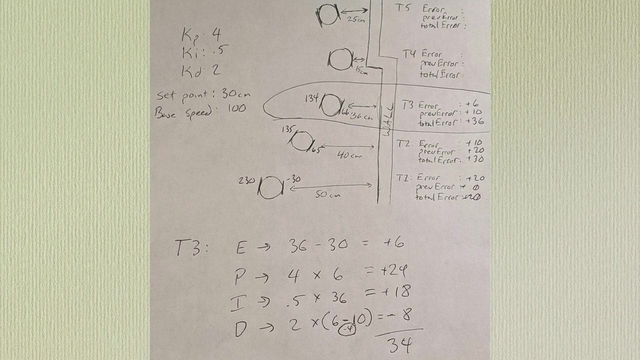 and this makes sense because the error has shrank. We would want our robot to be less aggressive as it approaches the set point to have less chance of overshooting it. Now that our robot is at time three and we're approaching our set point, we can see that our error, which is only six here, because 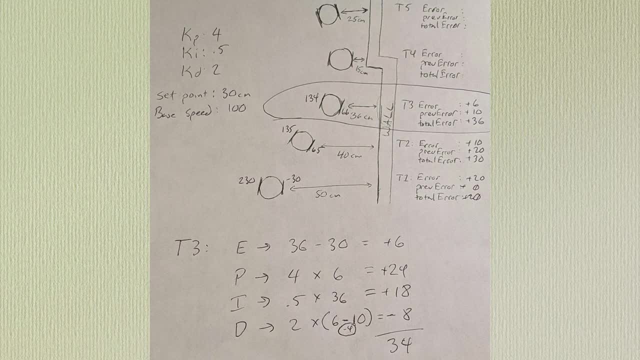 our robot is 36 centimeters from the wall is much smaller. Let's see how that plays out in our algorithm. So our proportional uses the same constant four times six, this time only producing 24.. Our integral does one half of the total, which, remember, used to be 30 because it was 20 plus 10. 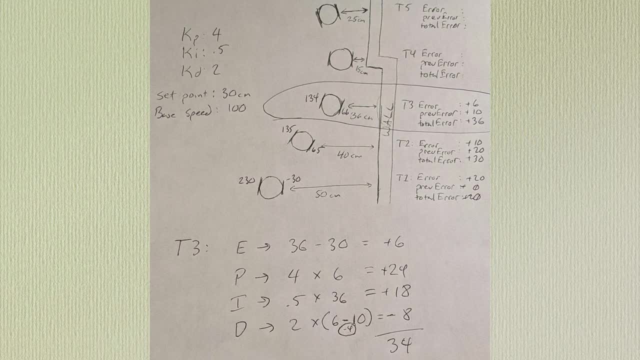 but now we took the 30 and we're approaching our set point. We can see that our error is only six here, because our robot is 36 centimeters from. the wall is much smaller. Let's see how that plays out. added in our six and our total is now 36.. So this is growing and this is going to keep. 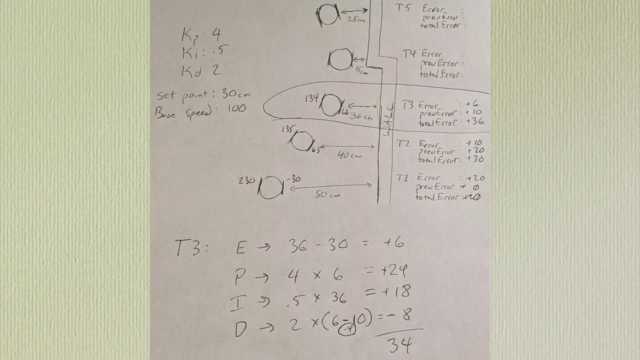 growing. This is an interesting property of integral, because we are totaling the error. the longer we stay on one side of the set point, the larger the integral is going to grow. So now we have an integral of positive 18.. Our derivative is now doing exactly what. 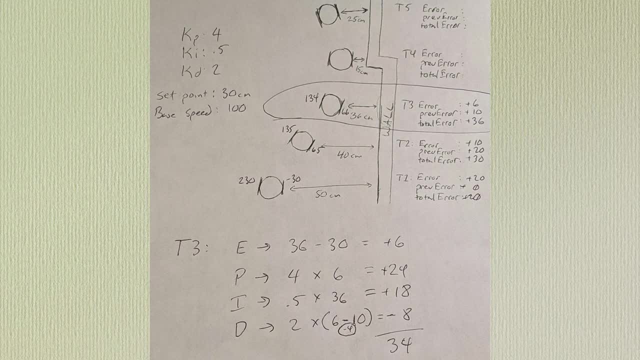 it should. it's acting as a buffer. so we have our constant of two and it's being multiplied by the difference of the current error of six and the previous error of 10, which is only a difference of four. So that gives us a negative eight. Again, this is acting as a counter pushing. 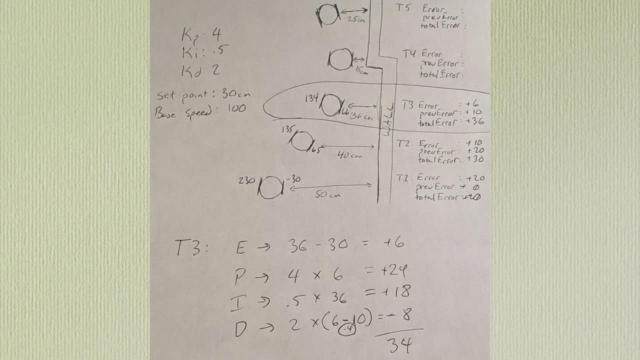 against the proportional and integral, Our total for our pit controller this round is 34.. Applying it to the wheels, you can see it's not much difference. We have a 134 and a 66 and we are still being pushed towards the wall. So we're still pushing towards the wall. We're still 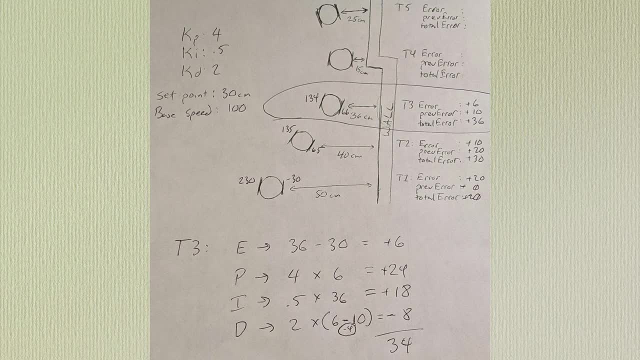 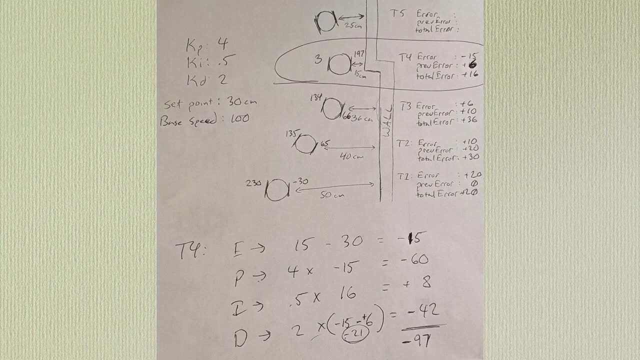 pushing towards the wall. Notice that the increased integral has helped push us more towards the wall and we haven't actually slowed ourselves down much At time. four: now the robot has met an interesting deviation in the wall. The wall actually has jutted out towards the robot. 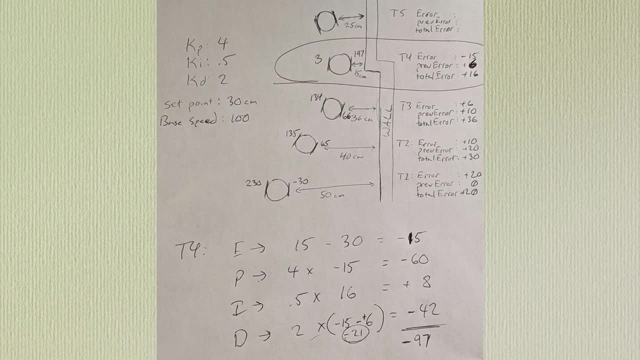 This could be just a simple change in the wall itself, or maybe there's a door or a molding, It doesn't much matter, I just wanted to throw a wrench in the works to give it some flavor. So at this point now our error has completely flipped because we are only 15. 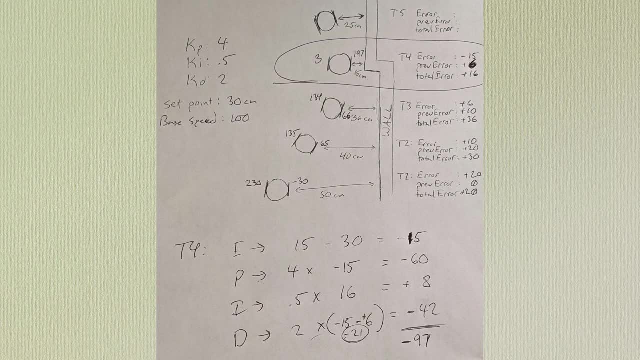 centimeters from the wall and we intended to be 30. We probably would have been close to it had this not happened. So our error is negative 15.. Putting this into our pig controller, we're going to have our constant 4 for proportional times, the negative 15, which gives us a negative 60.. 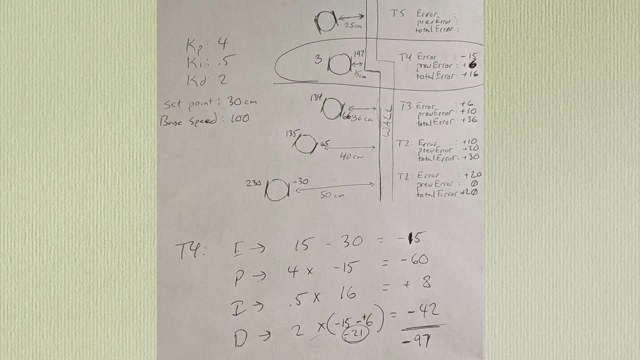 Our integral into, interestingly enough, is still positive, because the negative 15 error is added to the positive 36 that we used to have and that leaves us with a total error of 16.. Multiplying this by the 0.5 gives us a plus 8.. 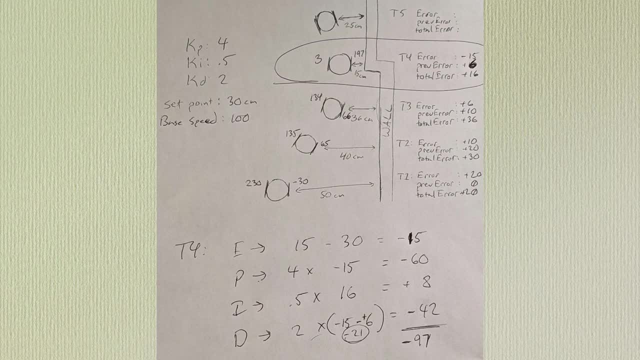 The derivative now is a positive 2, and it's multiplied by the difference of a negative 15 subtracted from a positive 6, which gives us a negative 21.. Now this, of course, is a negative 42. adding all this up, we get a negative 97, which does as we kind of hoped it would, since we're 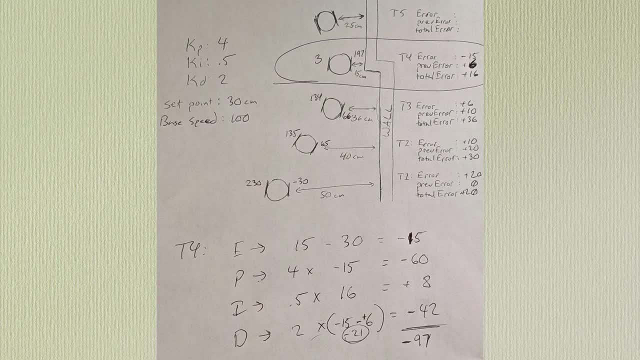 now pretty close to the wall, a pretty abrupt about face on the motors. On our right motor now we have a motor speed of 197 for the base speed plus the 97, and on the left wheel we have a 3.. Now remember, because we've gone over to the other direction of error, we have reversed the output on the motors. 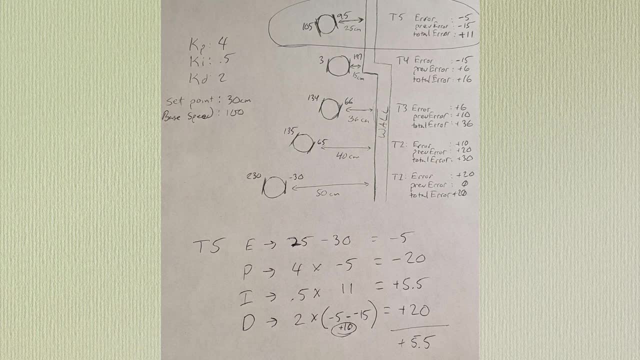 Time 5, our last time. now we can see that the robot has started moving back away from the wall. Currently we are 25 centimeters from the wall, which means we have an error of negative 5.. If we take this error and pop it into our PID, we can see that our proportional gives us a negative. 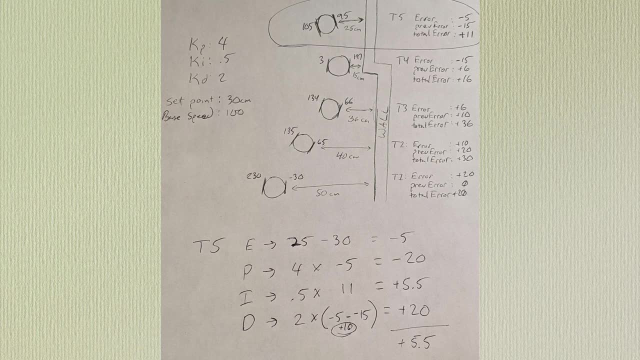 20 for 4 times negative 5.. Our integral is now still shrinking but, believe it or not, still pushing the robot back towards the wall because we had a pre-final error. So now we can see that our total error of negative 5 is about 5.5 and we'll be using that or rounding. 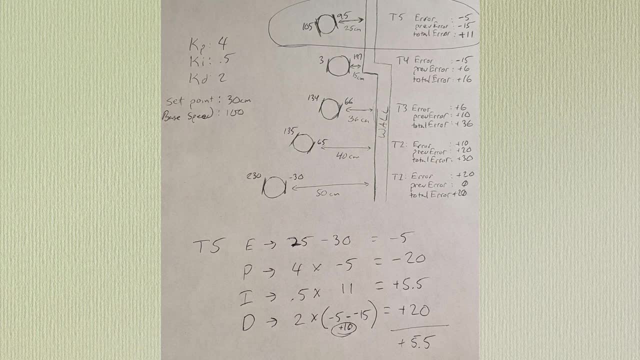 it. but you get the idea. The derivative is now going to correctly be buffering as well, so we have a 2 times the difference of negative 5, and subtracting that from negative 15 actually gives us a positive 10, so that gives us a positive 10.. Now we can see that our total error of negative 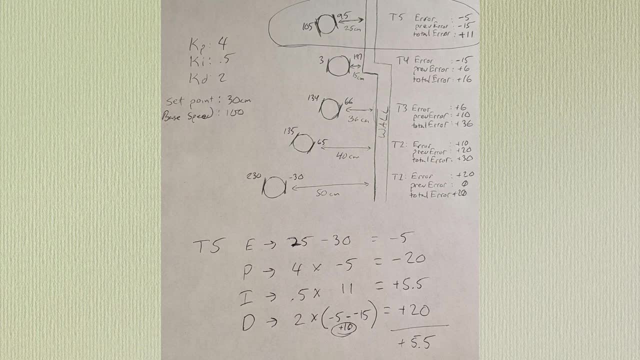 5 is about 5.5 and we'll be using that or rounding it, but you get the idea. Now notice: we have a problem here. The robot is actually being pushed a little bit back towards the wall As that integral shrinks. that will change and the robot will gradually stop being. 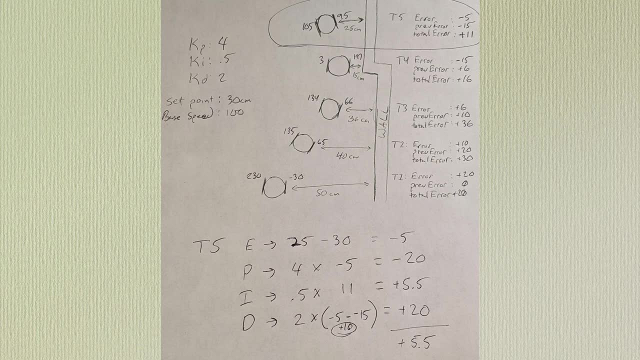 pushed back towards the wall, especially since the derivative won't have much change and that won't be affecting much either. But this is how you have to kind of play these things out, to really see how these three things affect it, so that when you think about the tuning and how much 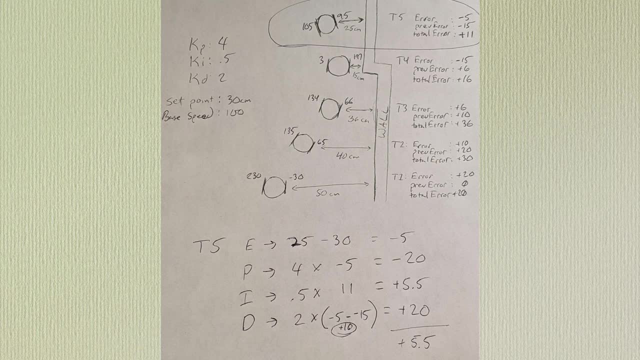 of a multiplier to apply to each, you can come up with a good result. What I highly recommend is starting with just one. Especially proportional is the one that is most often used. What I would do is start with a kp set a good number that seems to map well between your error and the. 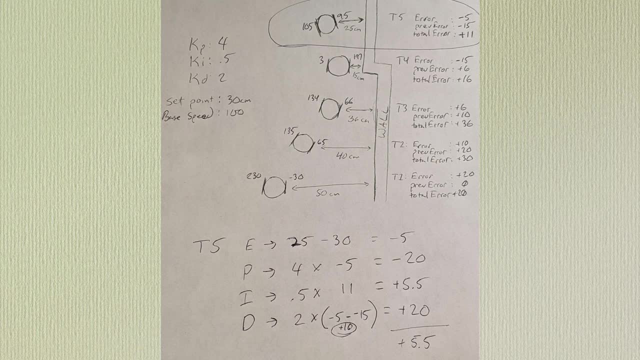 output, say of your motors, and then set your integral and derivative both to 0.. Once you have a kp that is in good shape, then move on and turn on one more of the parts of the PID. It's important to note that you don't need to use all three. 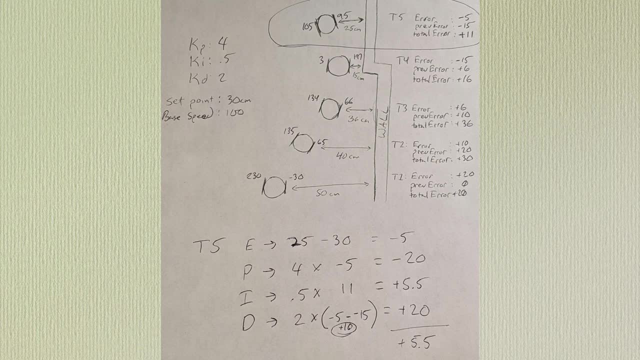 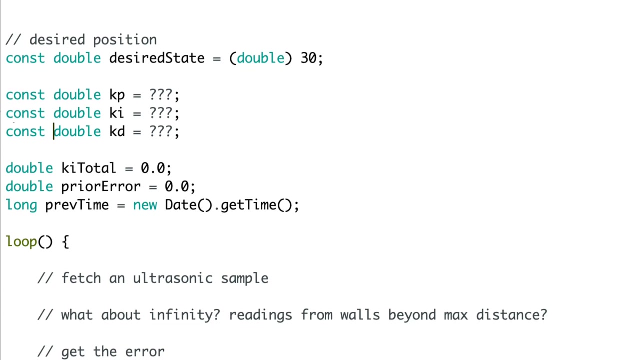 For some applications, like a robot that stands, all three are helpful, But for others, often like a wall following robot, you might not need all three. You might get by perfectly well with just kp, even, Or probably kt. I thought it would be useful to take a look at some pseudocode now that illustrates how you would. 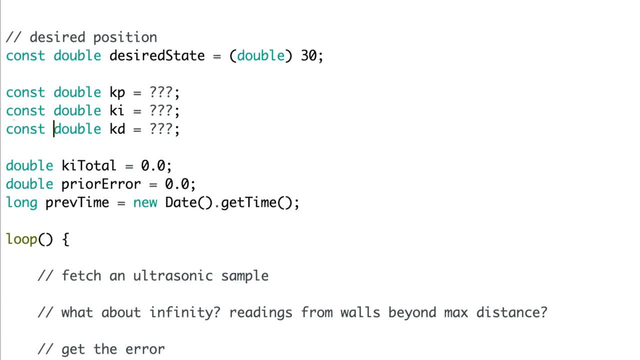 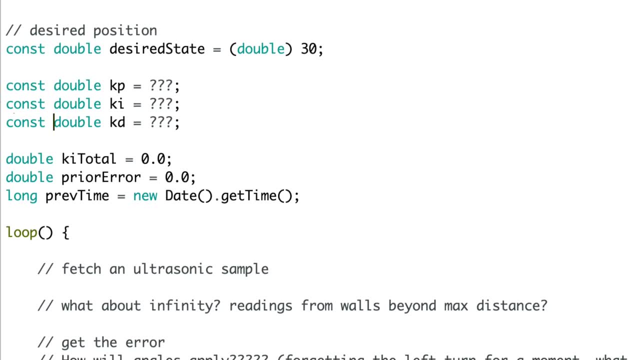 implement a PID. Now, this isn't meant to be a direct implementation. It's meant to be a layout, because every implementation is going to be slightly different, insofar as is your error positive or negative? If you're using a PID, you're going to want to make sure that you're 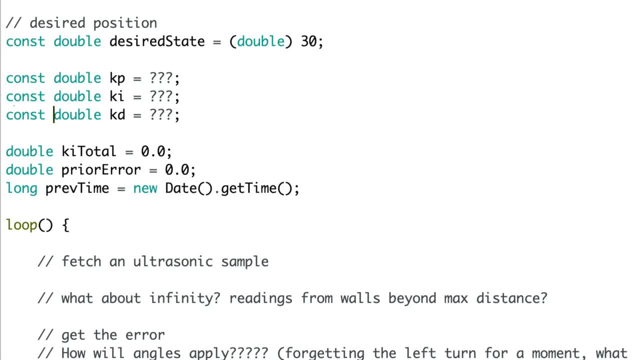 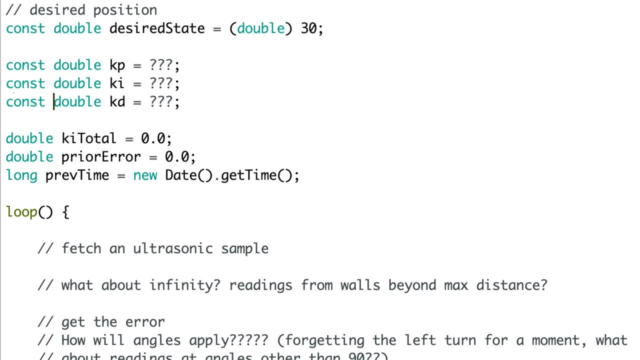 doing it in a way that's not negative, And how does that affect your motors and all of the little details? But the layout is the same. So I start up here with the desired state as a constant for a wall following robot. I kept with the theme and put it as 30. Then you have your three constants. 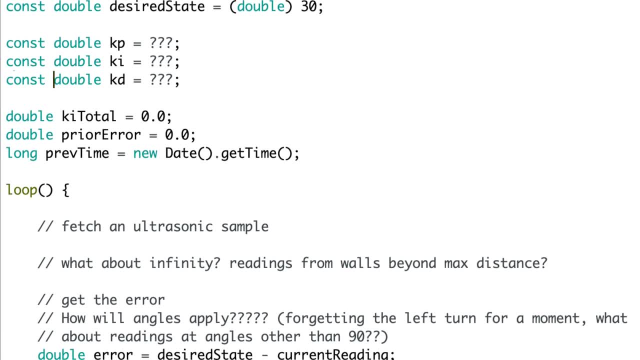 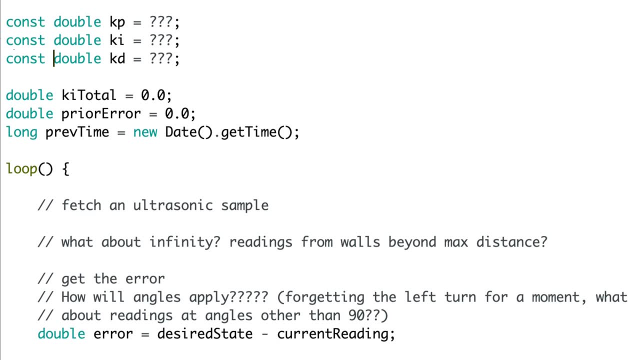 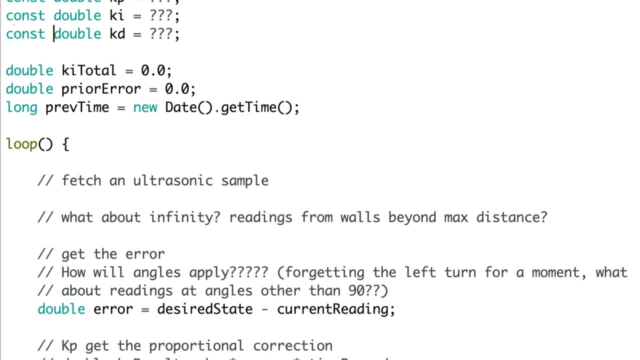 for kp, ki and kd. Remember these are your tuning constants. I highly recommend to start them at 0 and then do one at a time. Remember however much you put here affects the output of that part of the PID controller. We then also have our ki total and our prior error, The ki total. remember. 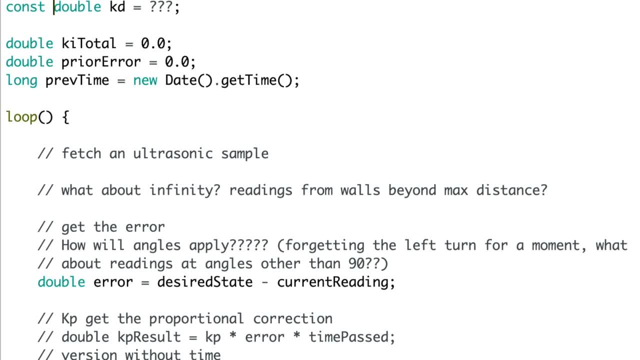 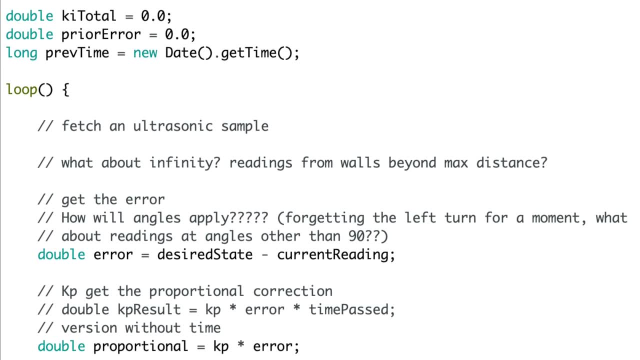 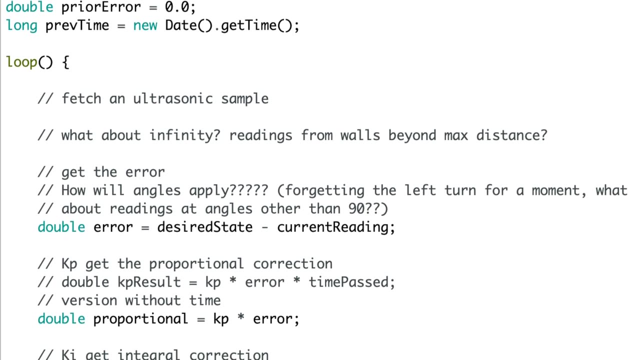 keeps track of the running total for the interval and the prior error keeps track of the prior error from the previous time. when you're dealing with your derivative, The previous time is in case you're using time. This would, of course, be optional and it's just initializing it. 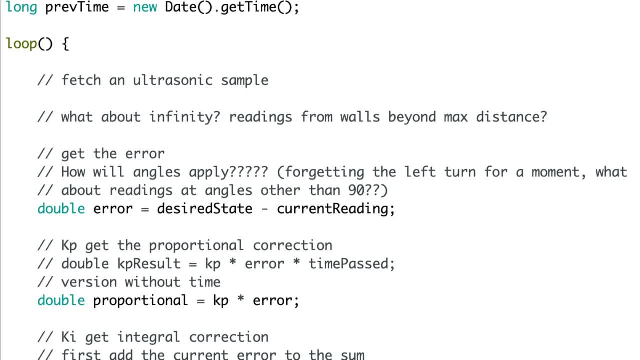 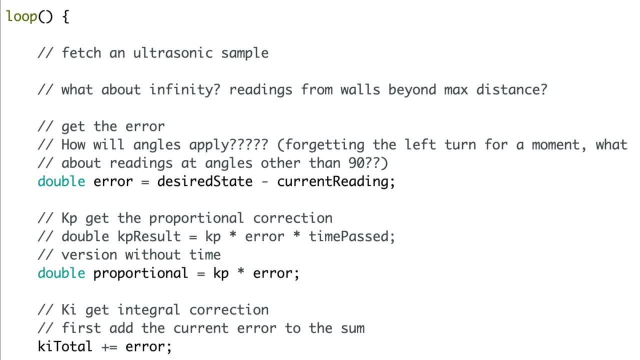 So once you're in the loop here, the first thing would be to get a sample. So this is a sample of whatever sensor data you're using to close the loop. Remember, this is a closed loop system and we're going to be comparing that sensor data to our set point And you want to. 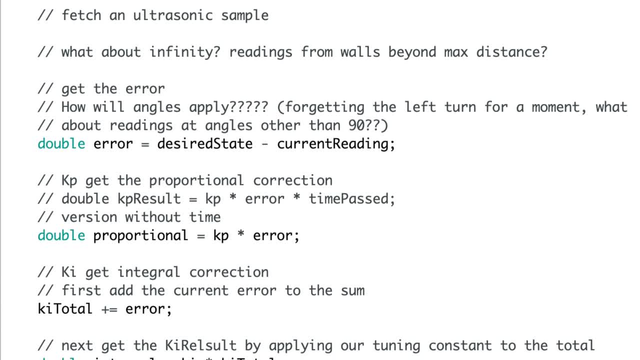 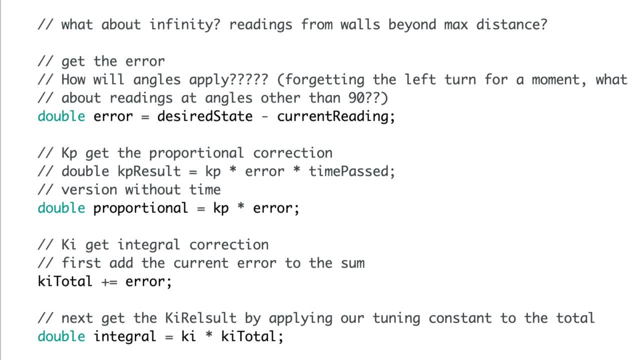 think about things like limits and make sure that you don't get infinity readings and things that are going to mess up your algorithm. Once all that's done and we've figured out what the error is by actually subtracting the current reading from the desired state, then we're going to start. 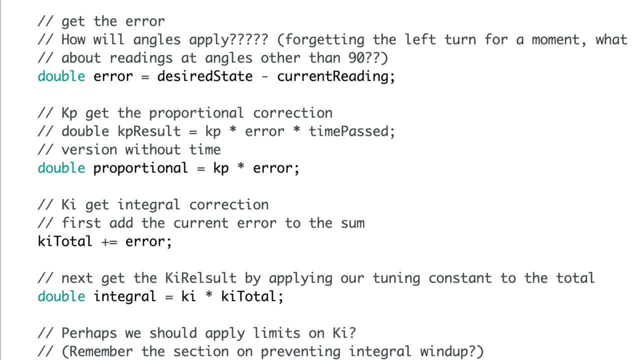 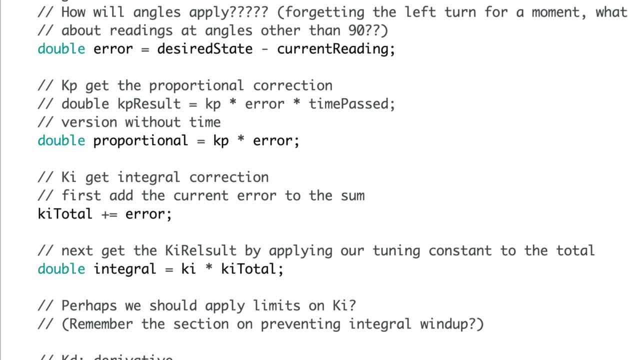 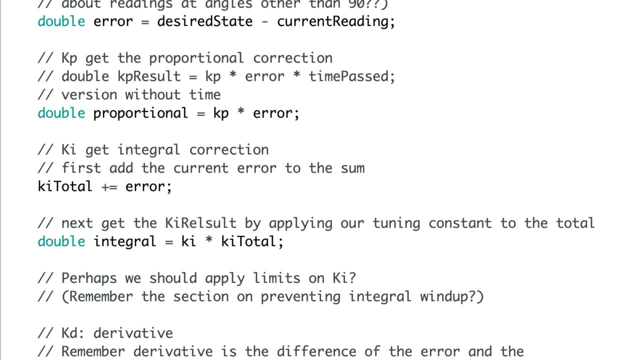 that error to our PID. So, starting with proportional, here we see that we just simply multiply the kp times the error. Now remember, if you are using time past, I have one commented out just above it. that also includes time. I've removed time for the integral and derivative. 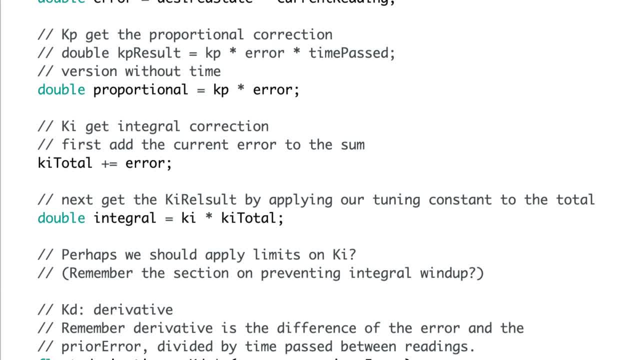 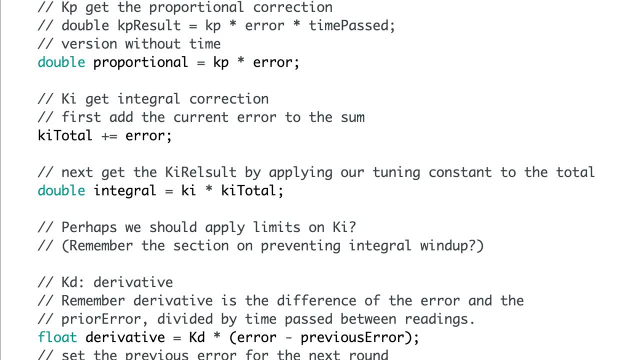 here as well For integral, the first thing we need to do is make sure that our running total keeps track of the current error as well. So here we are. We are adding that in. Then we simply multiply the running total also by the ki constant to get 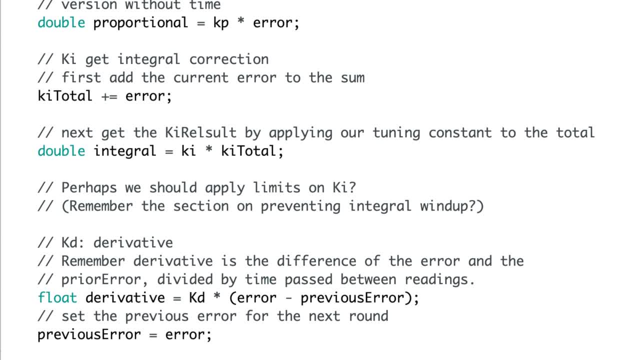 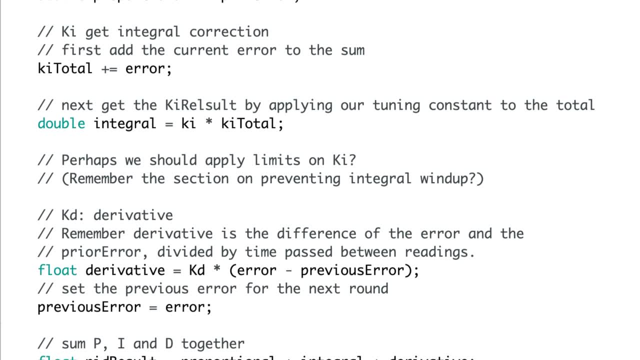 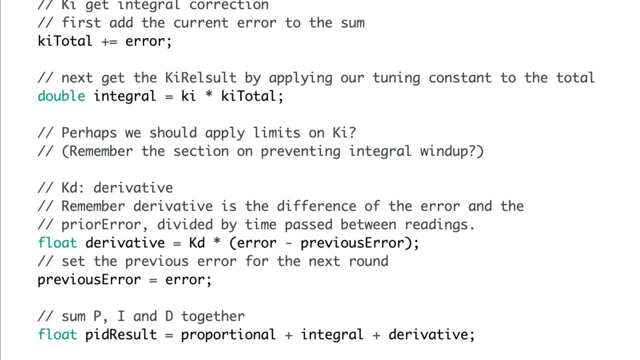 the integral value For derivative. we're, of course, taking our previous error and subtracting it from our error, multiplying it by our constant kd, and that gives us our derivative. Now we know, because we have to keep track of that previous error, that once we've done so, we should then 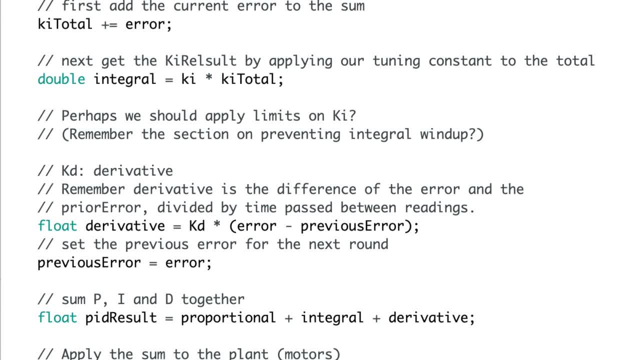 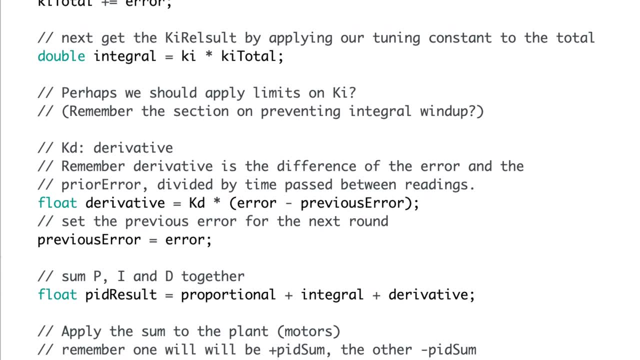 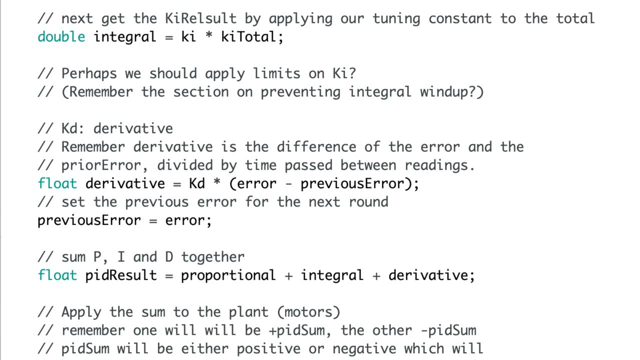 assign our current error to the previous error so that we have it for the next go. Now that we have all three pieces of the PID controller, we just simply sum them together to get the whole PID result. Now, please keep in mind that you do not have to use 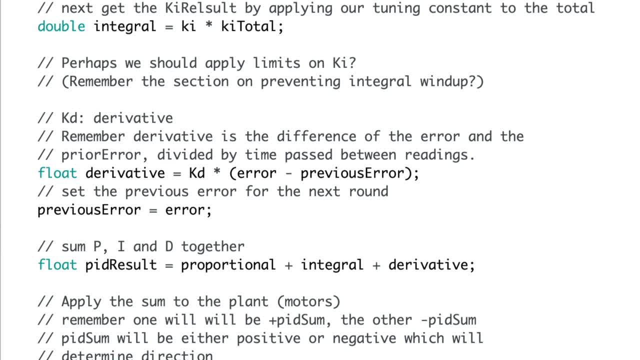 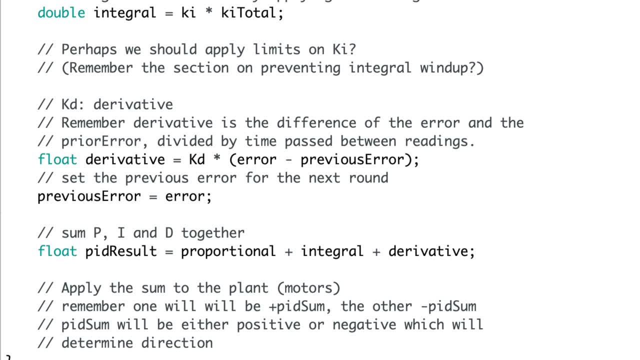 as I've mentioned before, all of the three. You can use proportional. you can use proportional and integral. you could use integral and derivative, although that would be a weird one. You can use any combination of the three, and when you do, you usually refer to it. 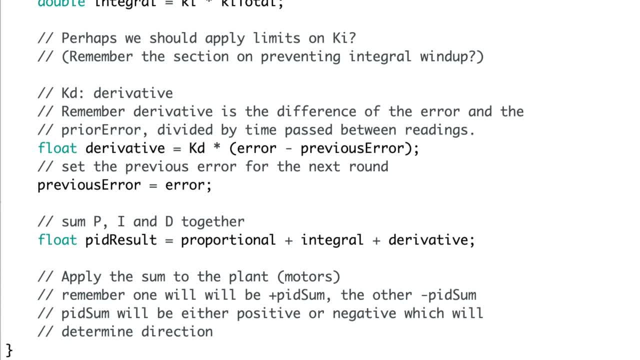 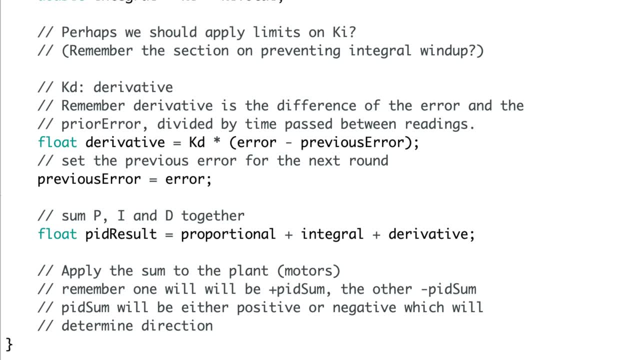 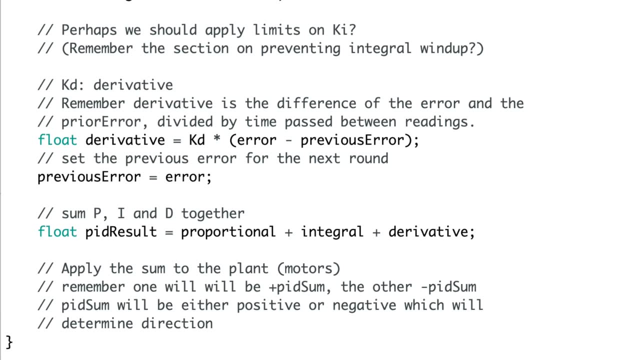 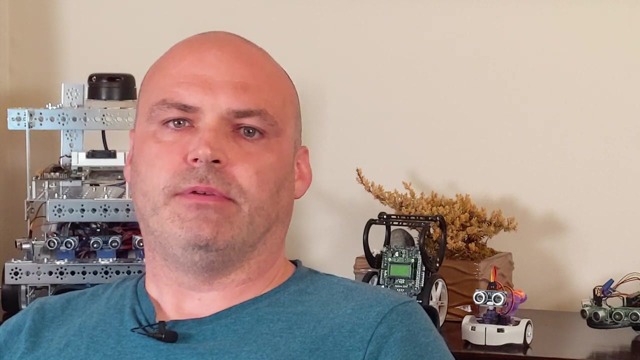 just with the kp times the error. So we're going to go ahead and do that. So that's everything we have time for in today's episode, but there is going to be more to come. on PID, I'm going to put together a video that is specifically targeted at how to tune PID. 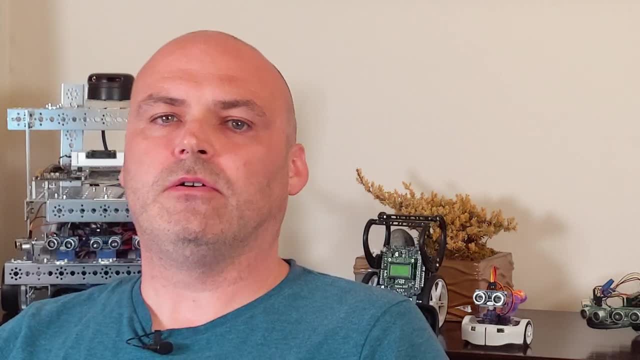 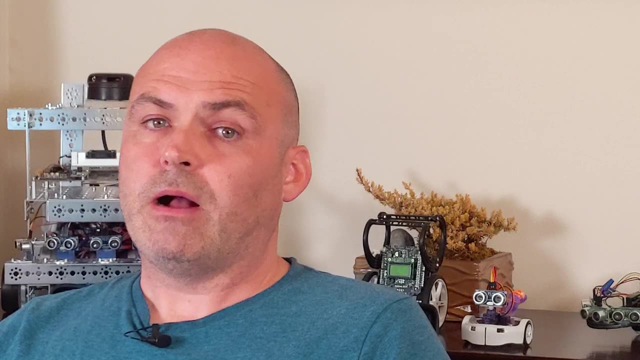 this is honestly an art form and it takes a long time to get used to the tuning. As I said, the math is easy but I didn't promise the tuning would be. Some problems are pretty easy. Doing a basic wall following isn't too bad.